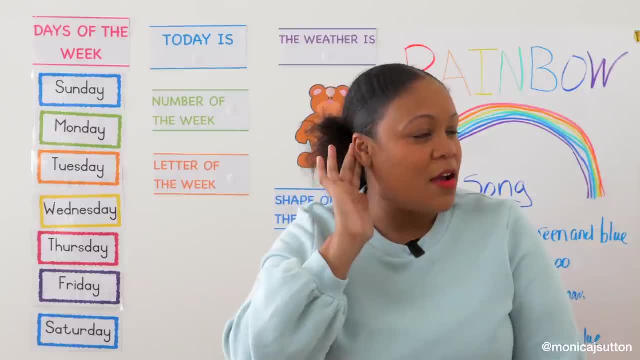 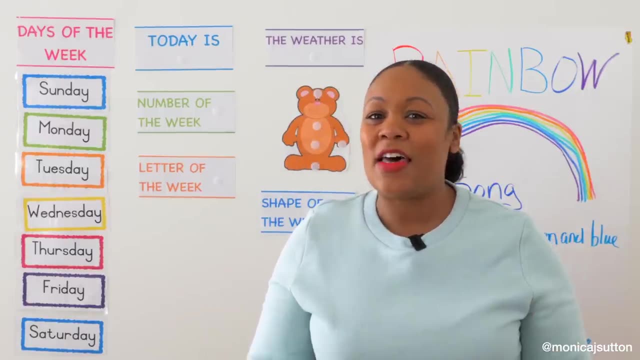 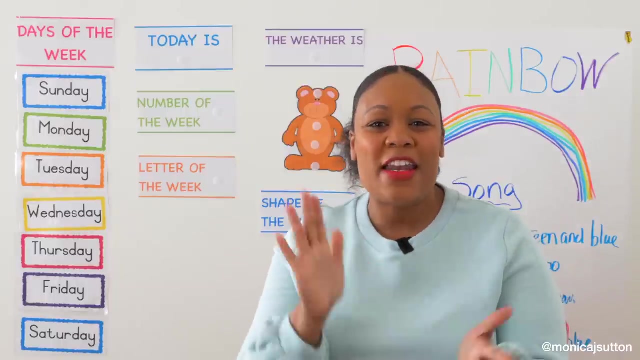 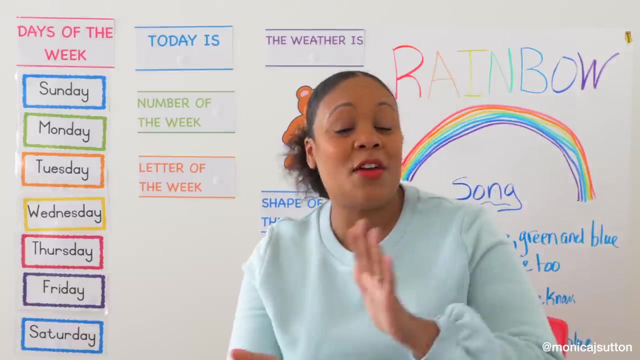 chugga choo choo. Listen, Is that our good morning train? I think it is. The good morning train is coming. How are you Choo choo? The good morning train is coming. How are you Choo choo? 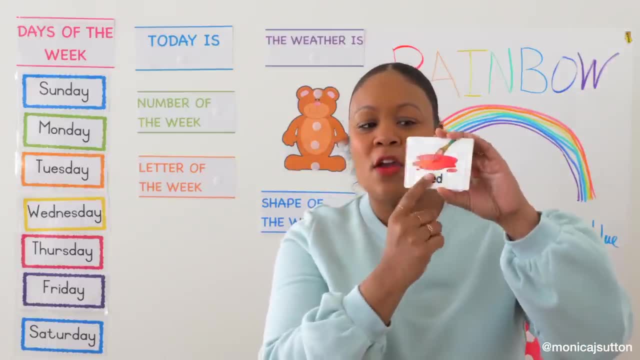 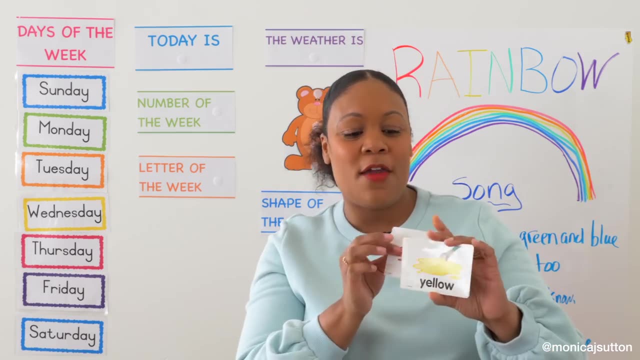 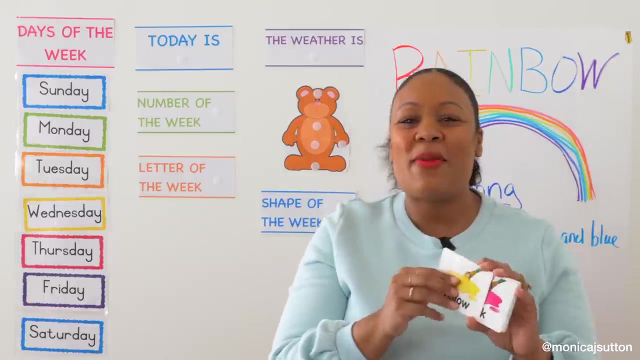 And we'll say hello to my friends wearing red. Are you wearing red Choo choo? And we'll say hello to my friends wearing What color? yellow, choo-choo. and we'll say hello to my friends, all my friends- wearing pink. 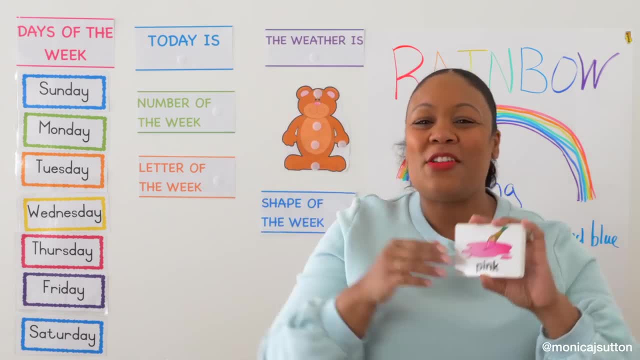 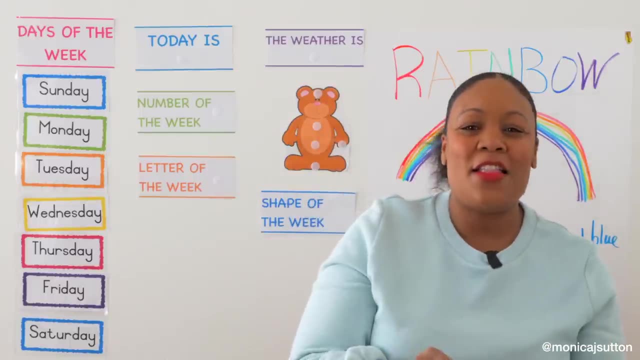 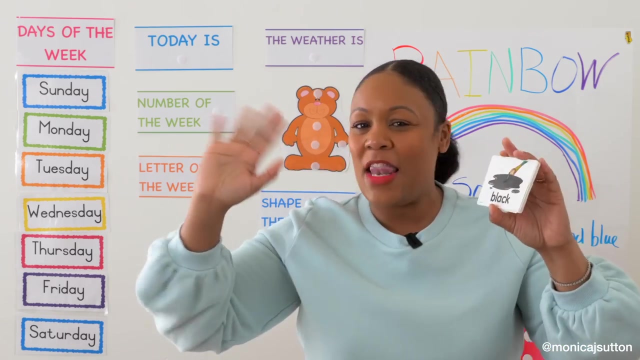 choo-choo, and we'll say hello to my friends wearing what color is that? can you see it? white choo-choo. and we'll say hello to my friends wearing green choo-choo. and we'll say hello to my friends, hello, friends wearing black choo-choo. and 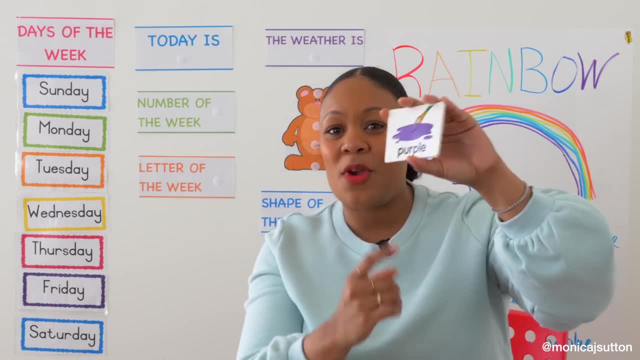 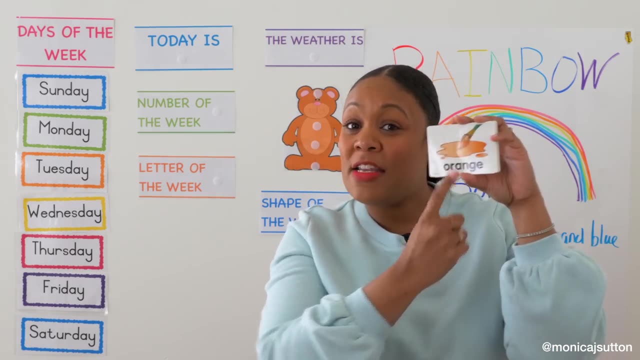 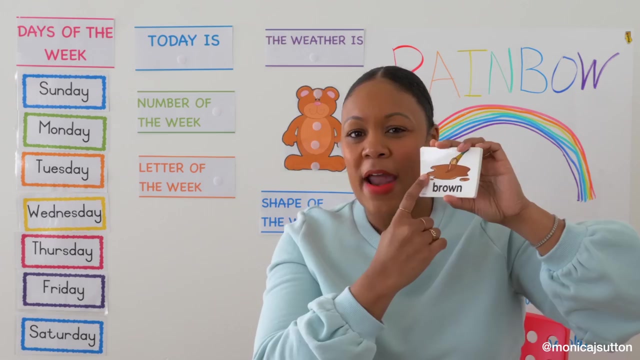 we'll say hello to my friends- all my friends- wearing purple choo-choo, and we'll say hello to my friends wearing orange choo-choo. and we'll say hello to my friends wearing what color is that? brown choo-choo. and we'll say hello to 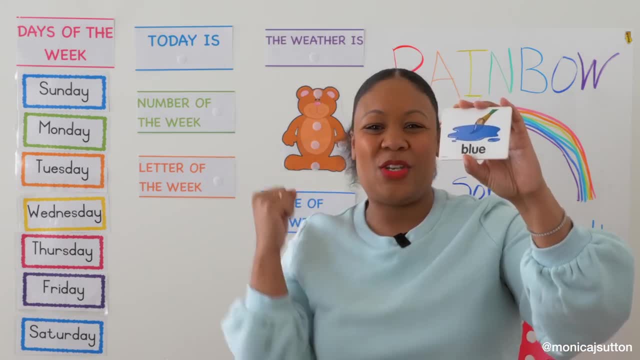 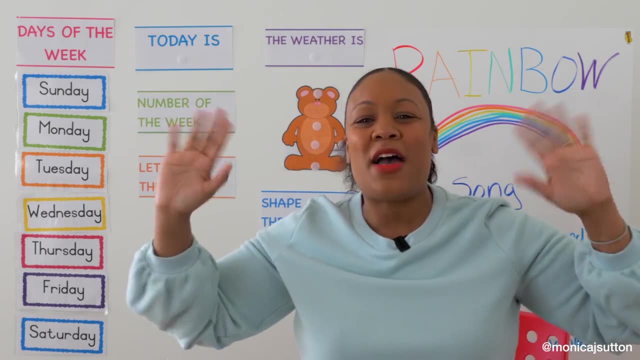 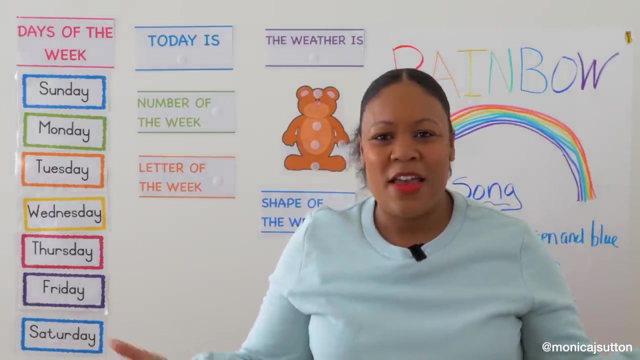 my friends wearing blue choo-choo and we'll say hello to my friends, all of my friends, and we'll say hello to everyone here in circle choo-choo. thank you everyone for singing our good morning song and I'm so happy the good morning train came alright, bye, good. 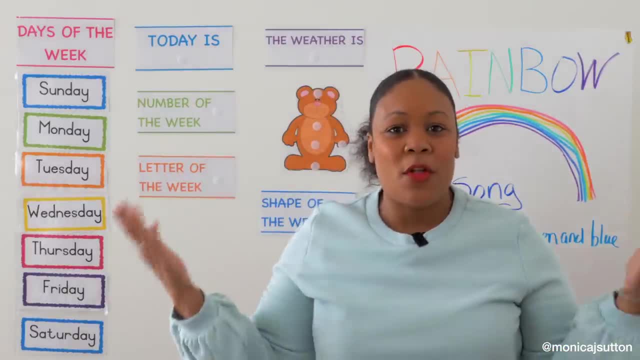 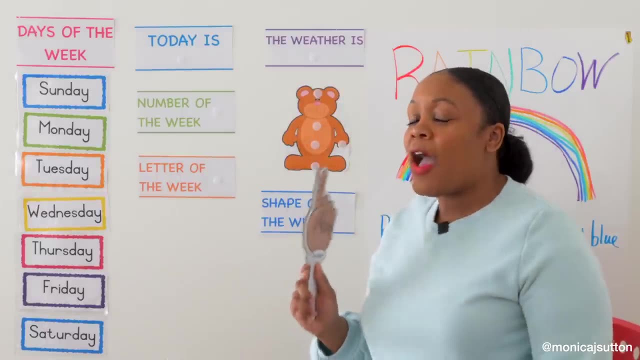 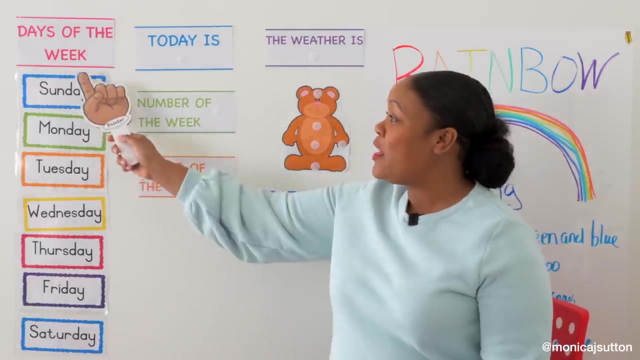 morning train. see you later. good morning train. now that we're all here, let's find out what day it is today. hmm, I'm going to use my pointer. by the way, I know that yesterday was Sunday, yesterday was Sunday, and so today is Monday. today is Monday, but 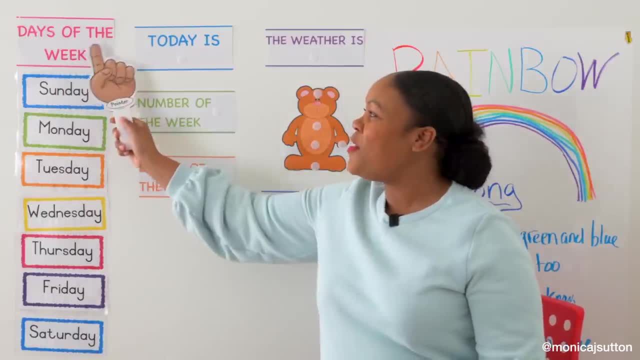 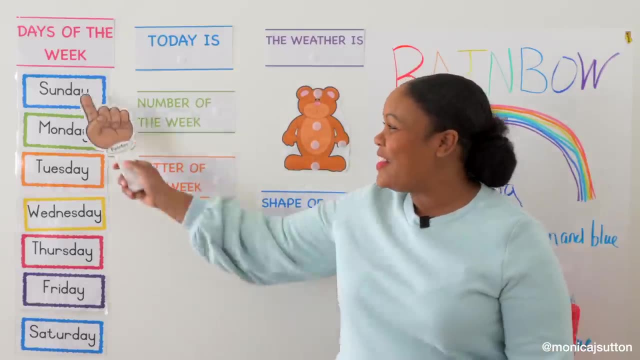 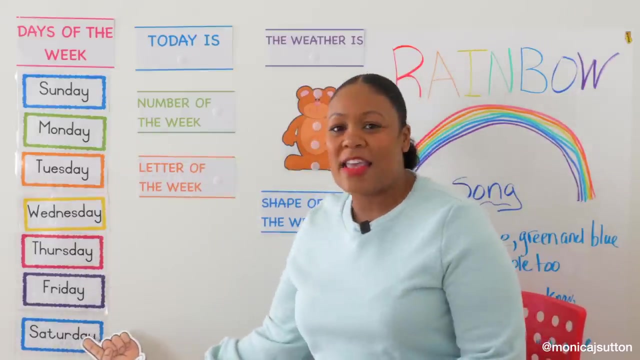 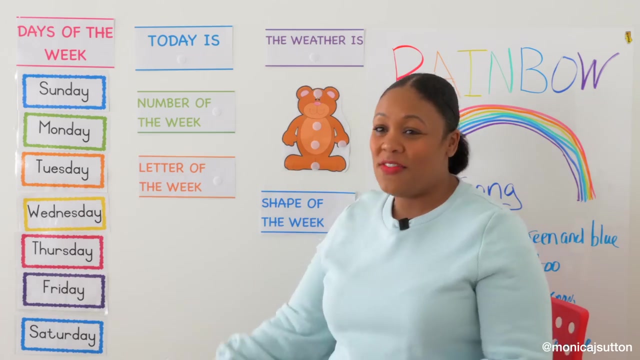 let's see all of the days of the week. can you sing with me? let's do it together this Sunday and this Monday, this Tuesday and this Wednesday, this Thursday and this Friday and then this Saturday days of the week. one more time there's such day. and this Monday, this Tuesday and this Wednesday. 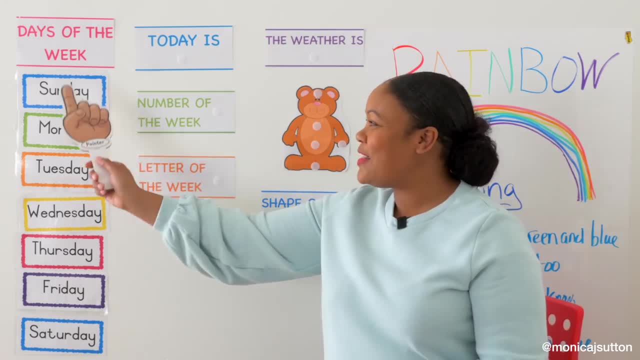 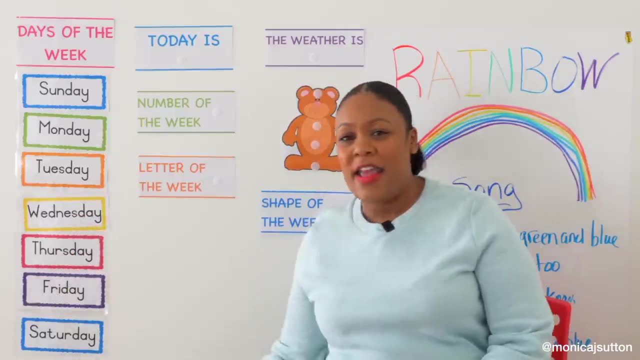 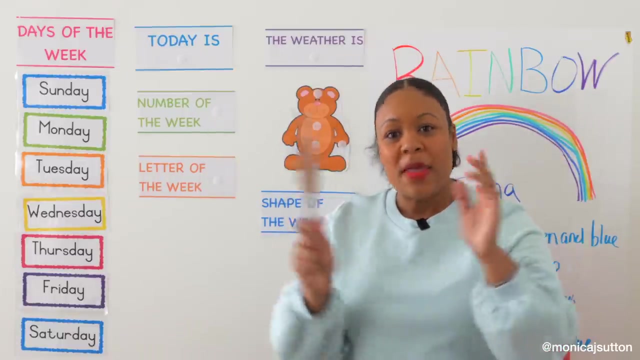 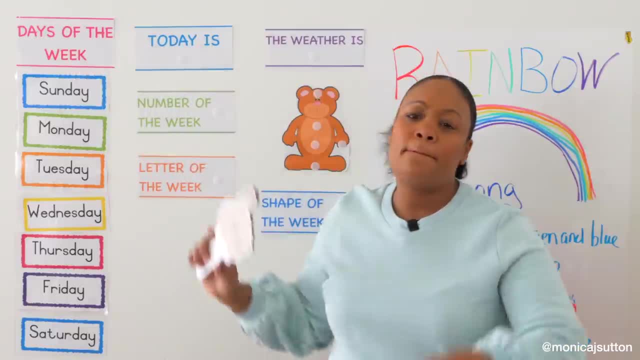 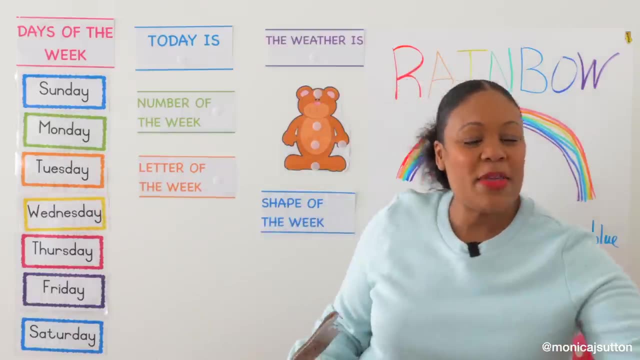 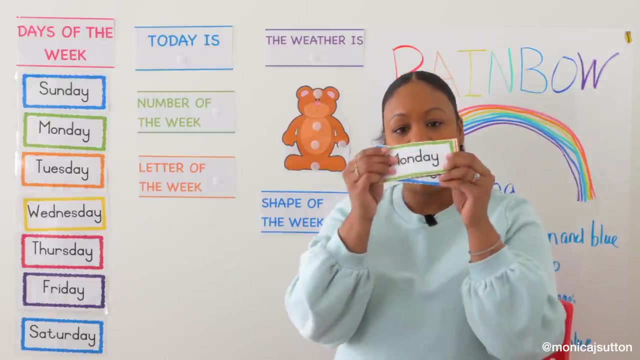 Rochester- unm怎么了, sorry, because I got a little bit scared. Sunday, so we say bye-bye to Sunday and today is Monday. today is Monday. now let me see if I can find Monday, because I have some smaller days. let's see if I can find Monday. oh there, it is right on top Monday. so we're going to take Monday. 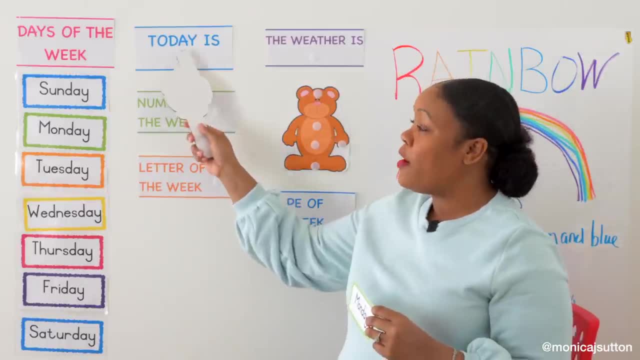 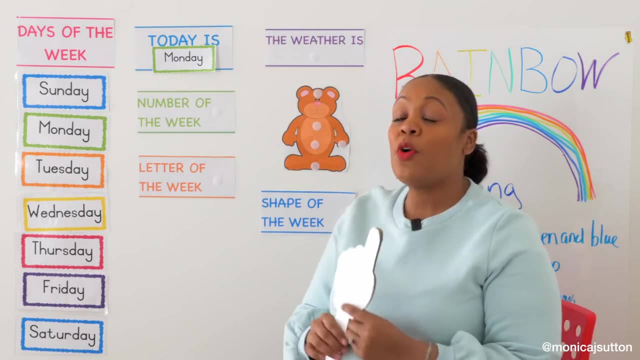 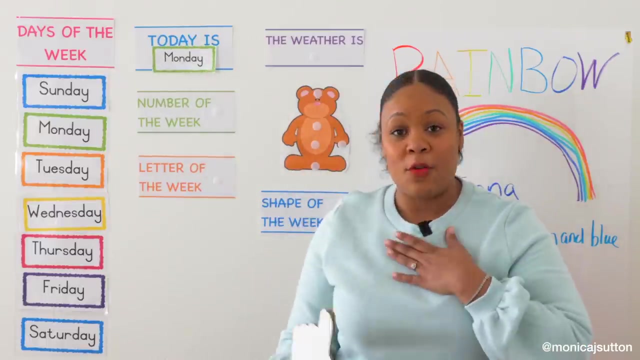 we're going to take this Monday and put it up here and hopefully you can say with me this sentence: let's say it together. first I'm going to put Monday and then we're going to read this sentence together. today is Monday, I'll read it first, then you read it second. today is Monday, your turn, let's read it. 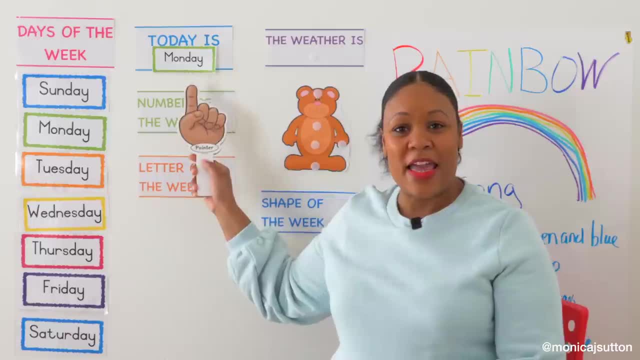 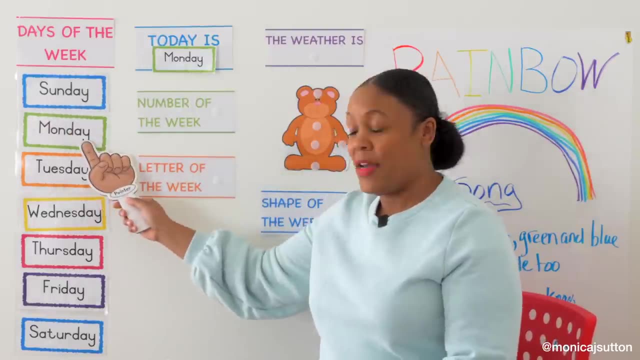 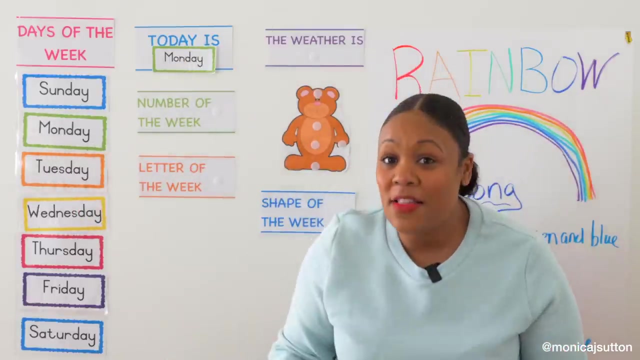 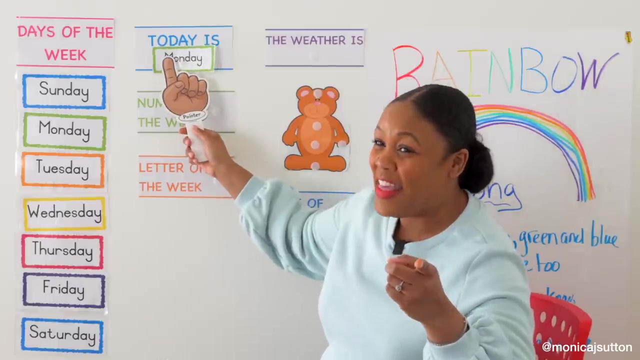 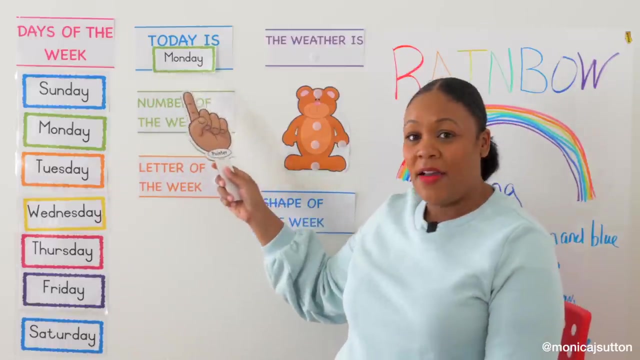 together. today is Monday, that's right. today is Monday. it's the day after Sunday, Sunday, Monday. today is Monday. today is Monday. today is Monday, all day long. today is Monday. today is Monday. today is Monday, that's right, all day long, all day long. today it will be Monday, Monday and I think that you can help me spell Monday. 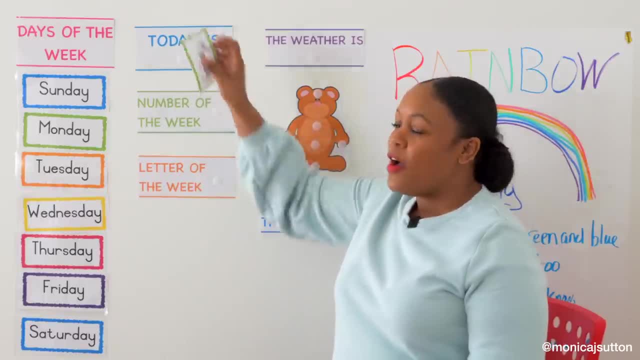 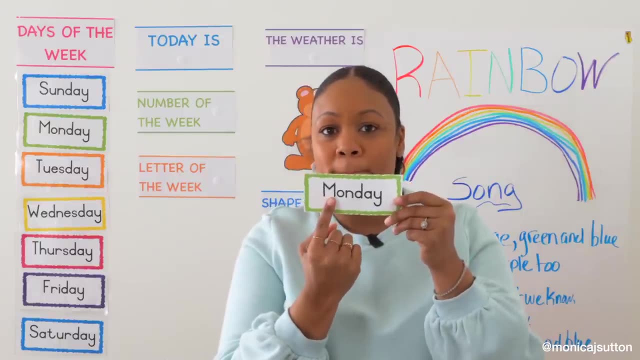 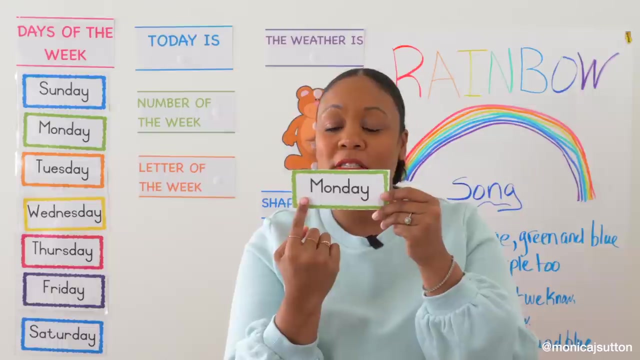 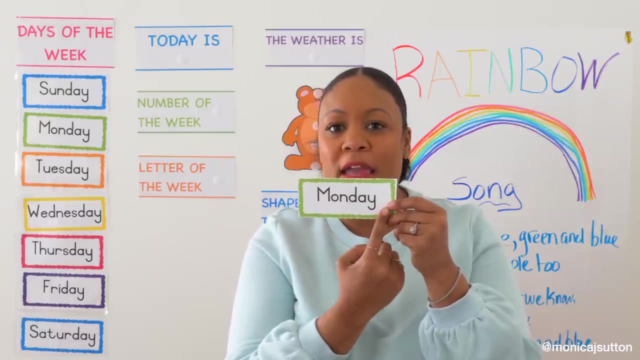 do you think you can help me spell it? let's spell it together. I'm going to take Monday off, so we can spell it together. our point and you spell with me: M O-N-D-A-Y. That spells Monday, and Monday starts with M- M for Monday. let's spell it one more time together: M O-N-D-A-Y. 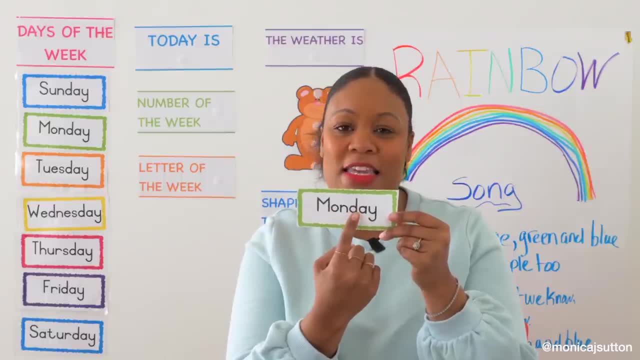 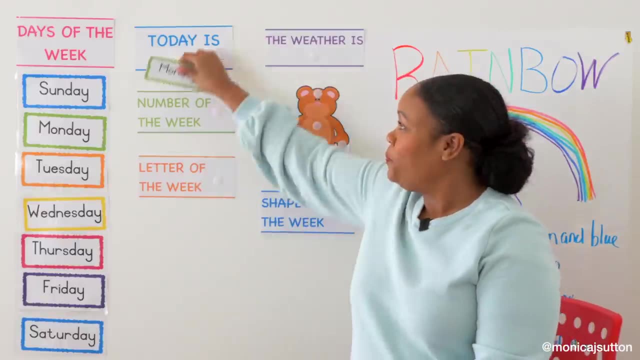 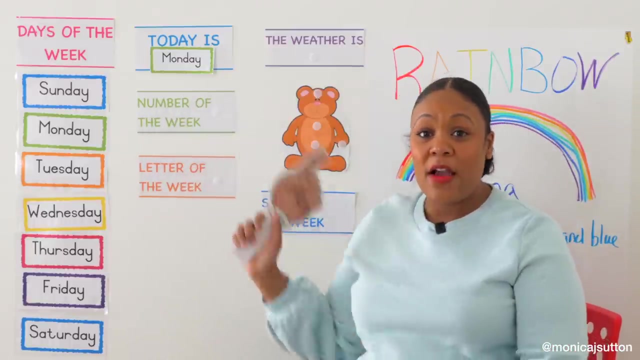 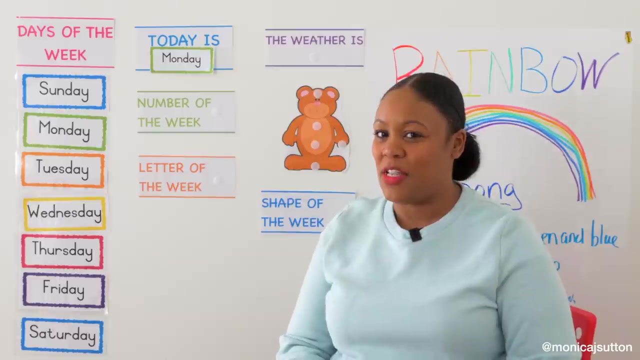 M O-N-D-A-Y. Monday- Monday, Let's put it back. Today is Monday. Okay, what's next? Next we have our number of the week. This week, we are going to talk about the number. Let me get it. Let's see who knows this number. We are going to talk about the number. Who? 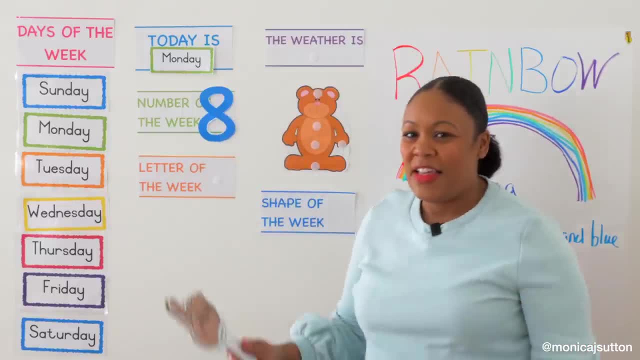 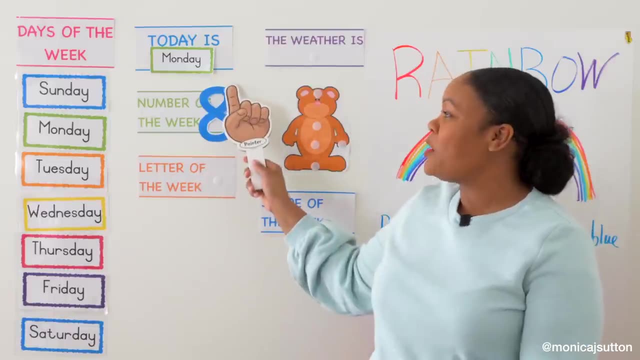 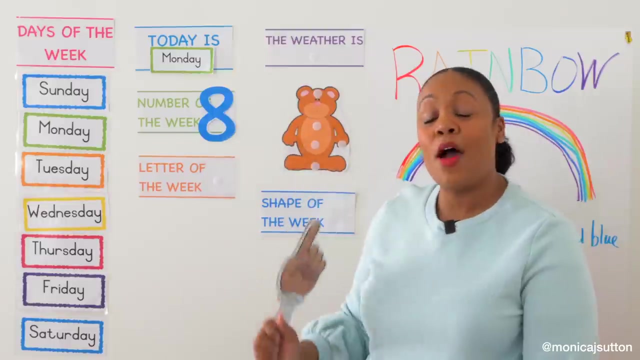 knows what number that is. Do you know what number that is? This is number eight Eight. Eight looks almost like two circles, one on top of the other, Almost right. It looks like two circles almost Eight. Number eight, That's our number of. 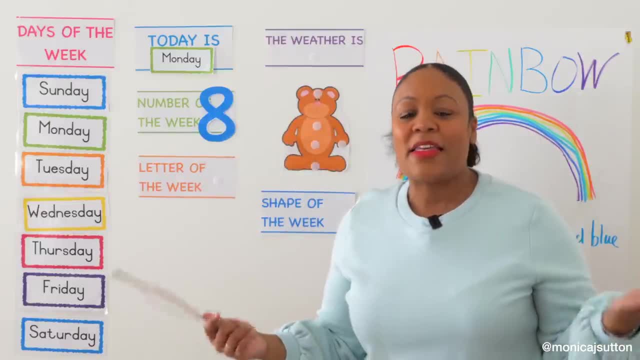 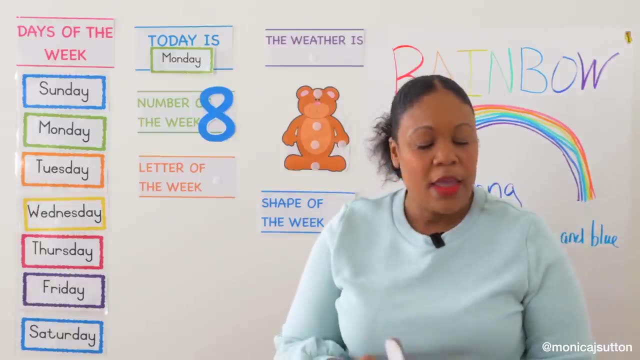 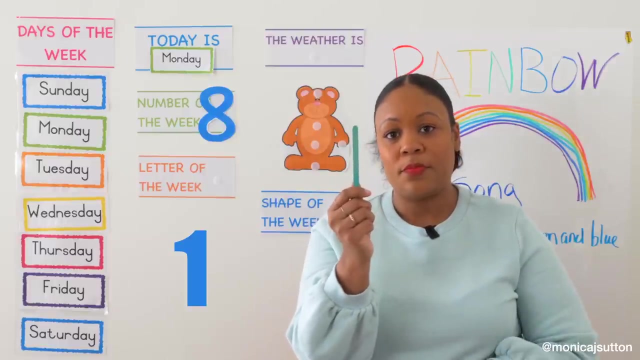 the week And I would love it if you would help me count to eight. I have these special, special sticks and I would love it if you would help me count my sticks. Let's see if I can count eight sticks. Are you ready? Okay, let's do it together, Starting with number one, Two, Let's keep. 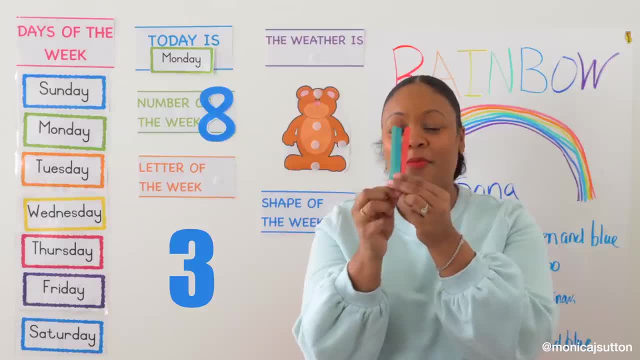 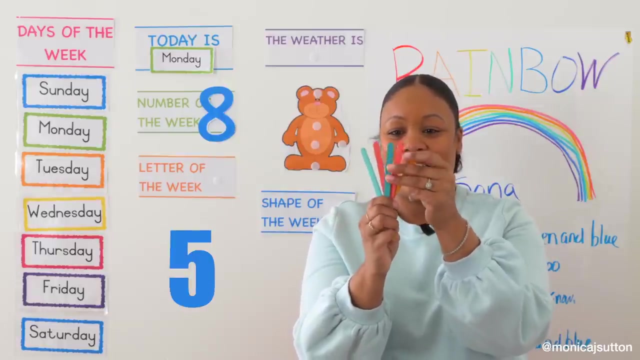 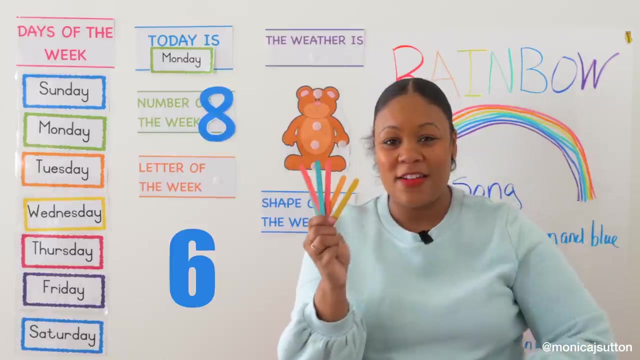 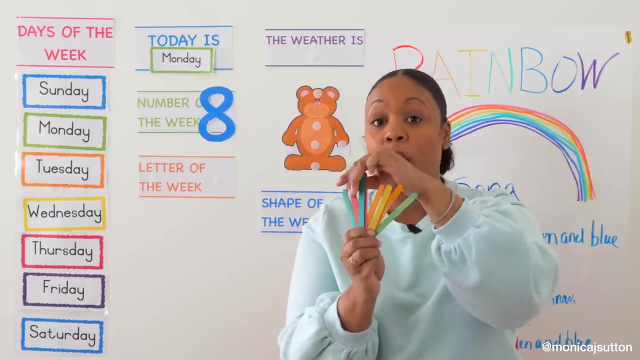 counting Three, Four, We're up to four now. That's four, Five. Oh, I think I have five now. Spread those out. Six, Six sticks so far. Seven, Eight, Eight sticks. Now let's count them one more time. Our number of the week is: 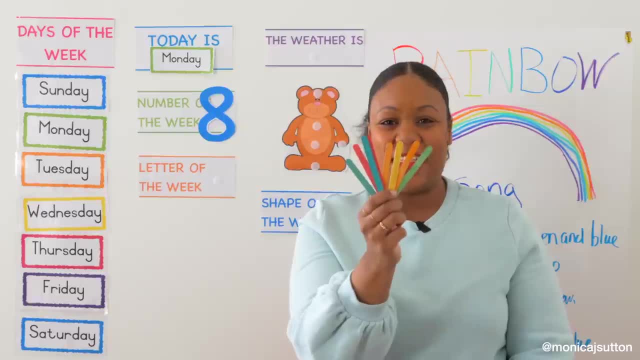 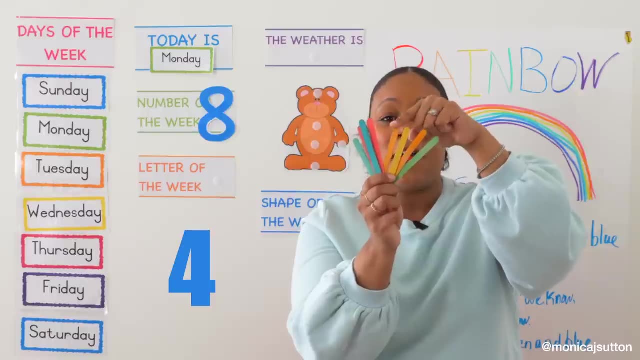 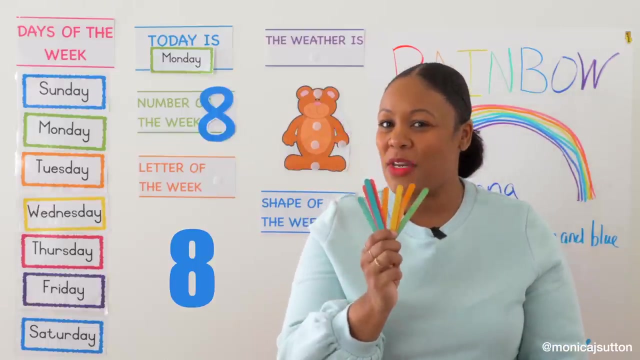 eight. Let's see if I have eight sticks. Count with me One, two, three, four, five, six, seven, eight. Do we have eight sticks? I think we do. You did it. Thanks for helping me count. 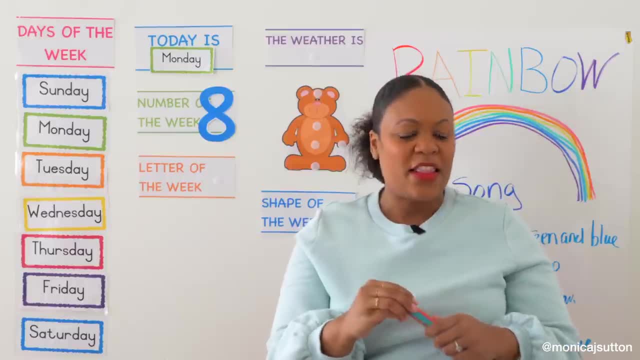 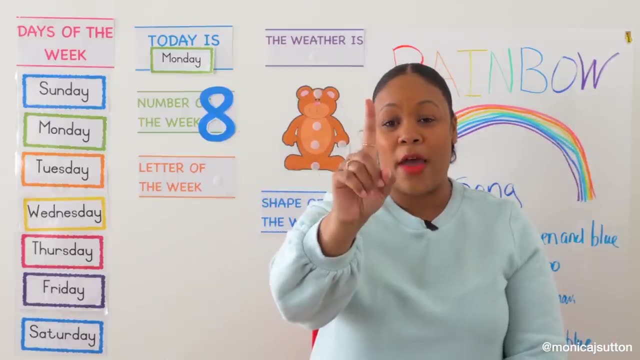 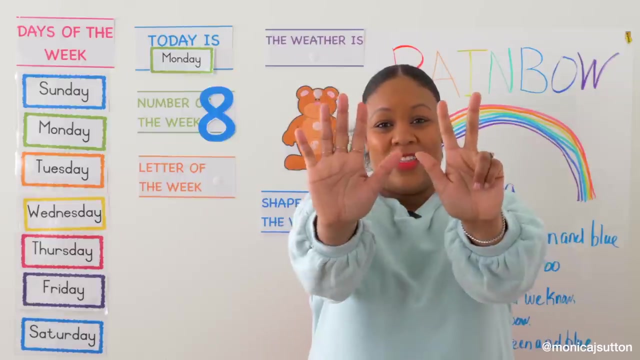 Eight sticks. Eight is our number of the week. Let's try counting eight using our fingers. Are you ready? Let's start with one, two, three, four, five, six, seven, eight. There are eight fingers. Did you count eight fingers? 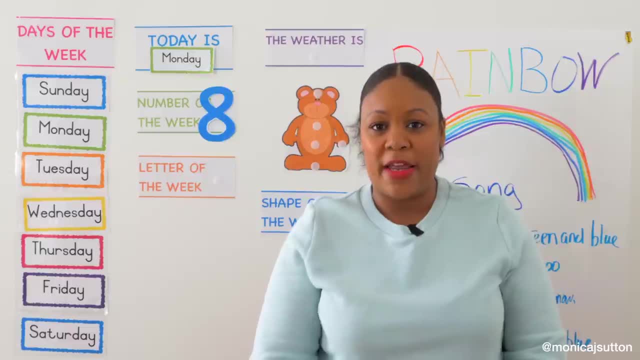 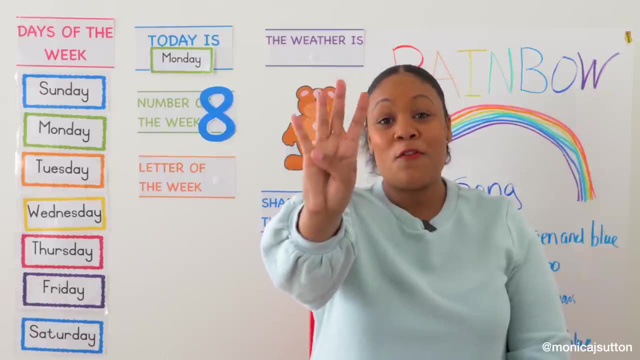 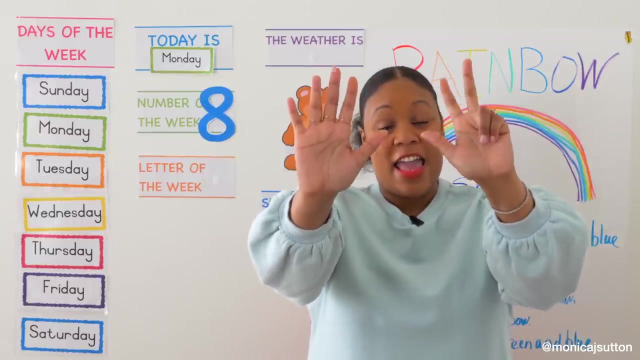 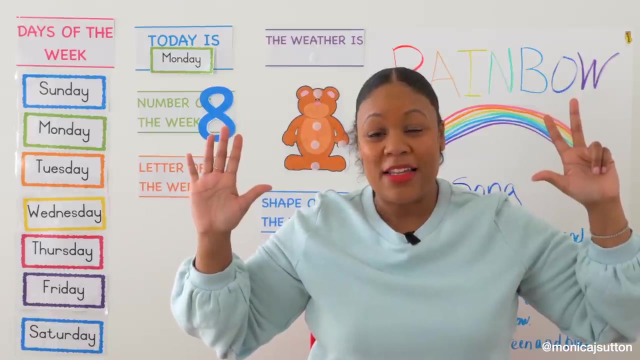 Let's do it one more time, Ready Together, Together One, two, three, four, five, six, seven and eight Eight fingers. I'm holding up eight fingers, Were you able to do it? Good trying. 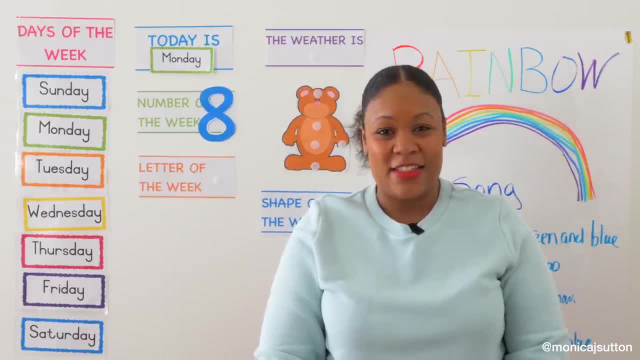 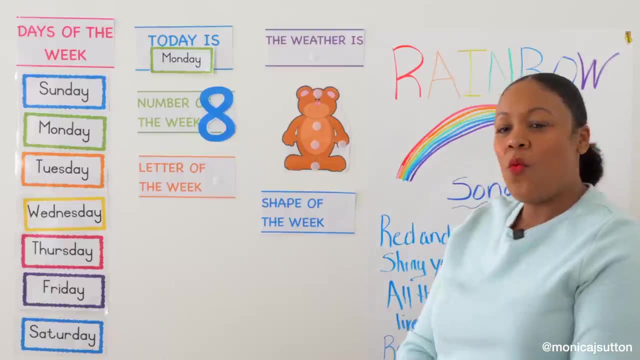 Eight fingers, The number eight. Really really good trying. Thank you so much for doing it. Stay with me Now let's see What is our letter of the week. Hmm, What letter of the week are we going to talk about this week? 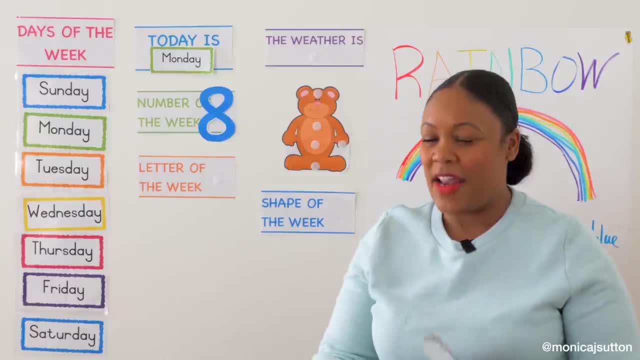 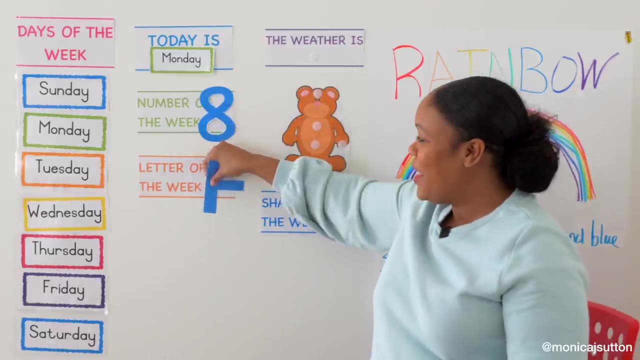 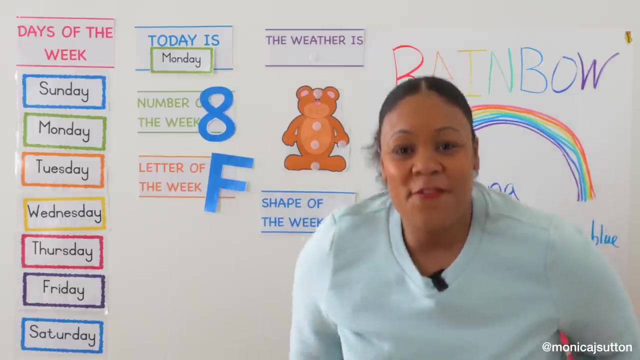 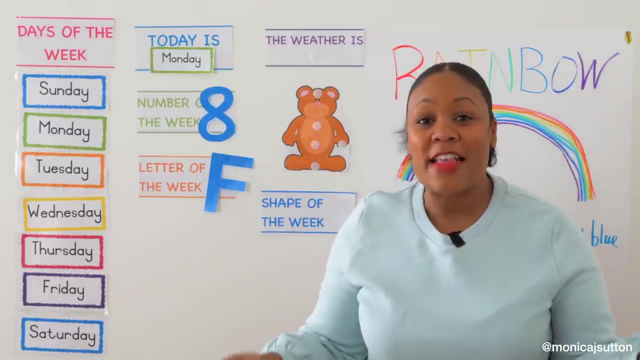 Let me show you the letter and let's find out Who knows what letter this is. The letter of the week is F, Letter F, F. F says F. F says F. Every letter has a sound and F says F. Can you do that? 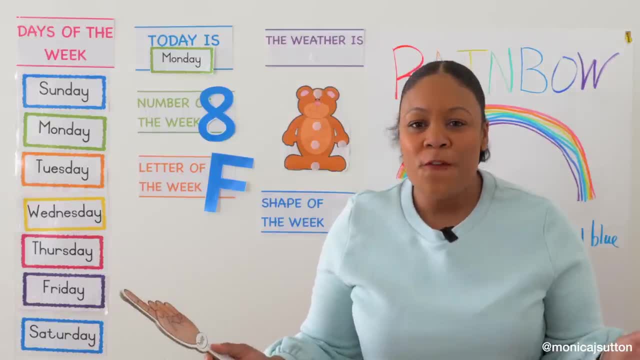 Can you make that sound with your mouth? F says F. If you put the top of your teeth on your lip, on your bottom lip, and go F, F, F, You can make that sound. F says F, F, F, F. 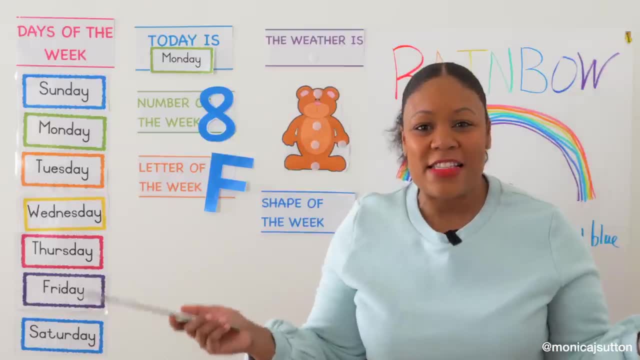 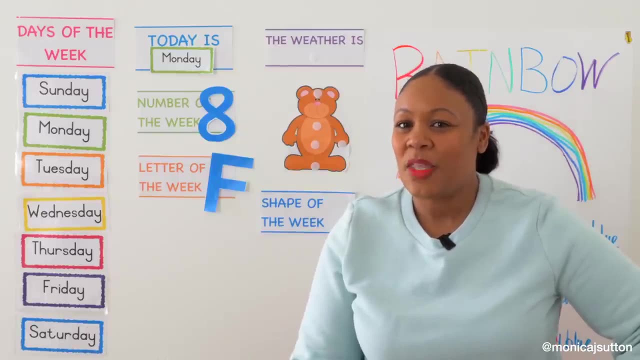 F says F, F, F, F. Every letter has a sound and F says F. Were you able to make that sound? Good, try, Very good, try. F says F. I wonder if I can think of some things that start with the letter F. 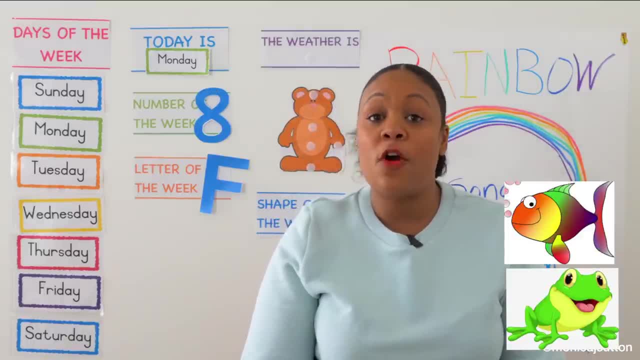 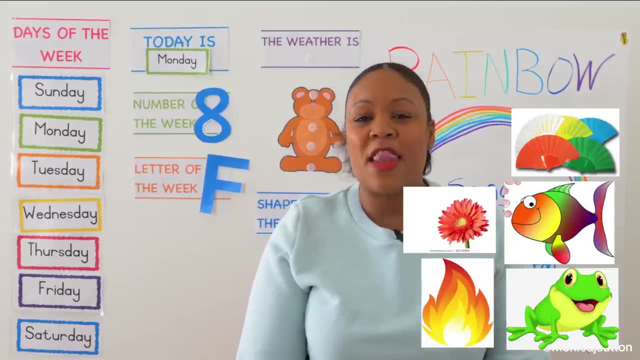 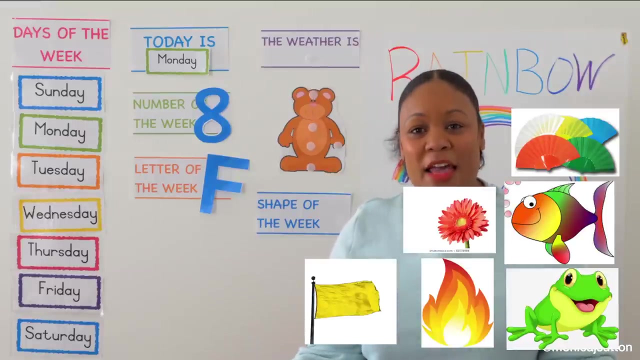 F for frog, F for fish, F for fan, F for fire, F for flower, F for flower, F for flag. That's the letter F. Wow, Thank you for sounding out those words with me. Letter F: All of those words start with the letter F. 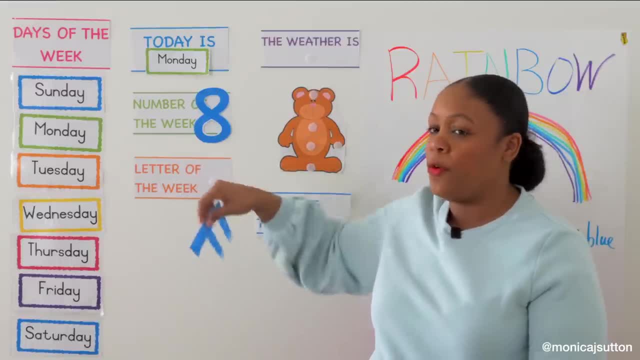 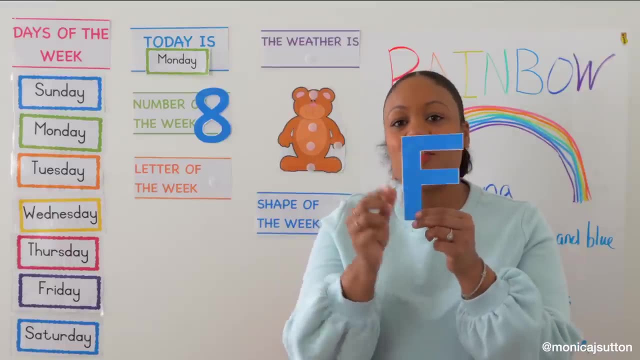 F is really special. Now I'm going to take F off of our board and hold it up so you can see it again, And this time I want us to use our pointer finger. Can you get your pointer finger? You just hold up one finger. 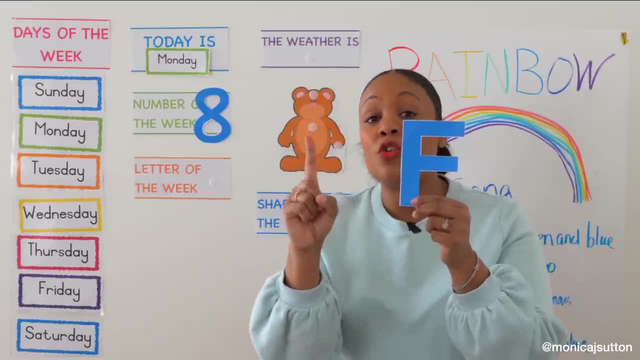 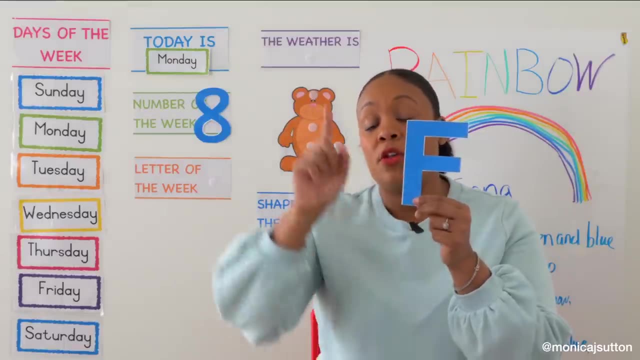 This pointer finger. Hold it up And we're going to use it to trace the letter F. Now you pretend you have a letter F and you can trace it right along with me. So hold up your pointer finger And we're going to start at the top of letter F. 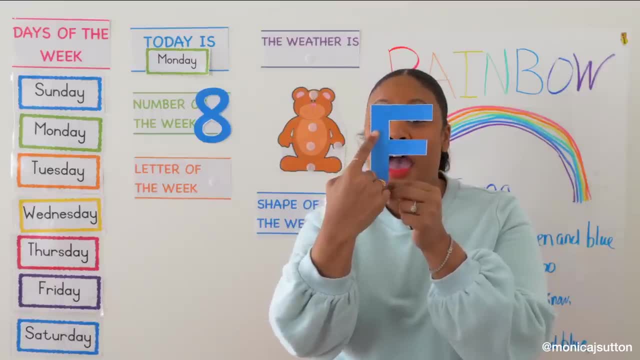 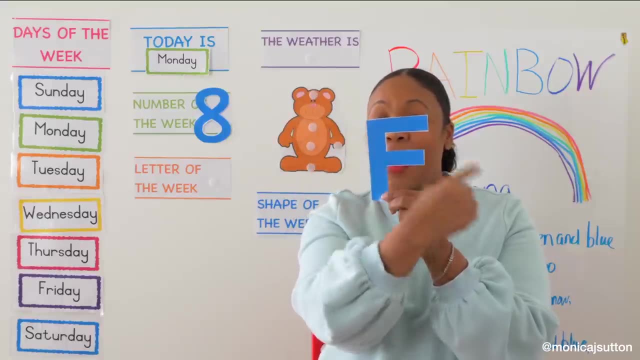 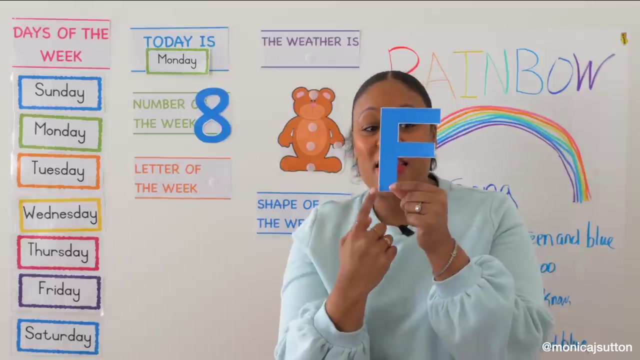 And go down- Stop. Then take our pointer back to the top and go across- Stop. And then take our pointer finger to the middle and go across- Stop. And that's the letter F. Now let's do it a little bit faster. 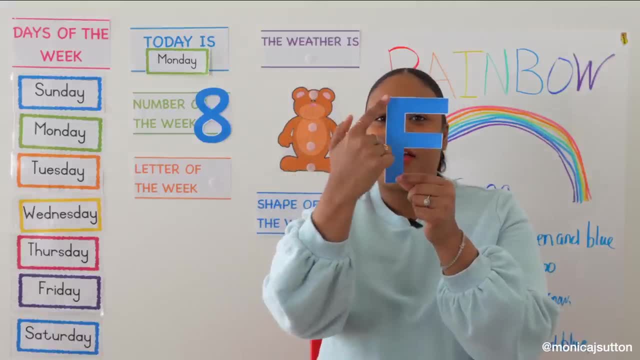 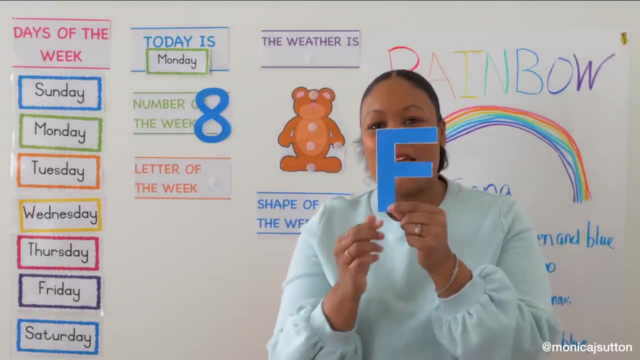 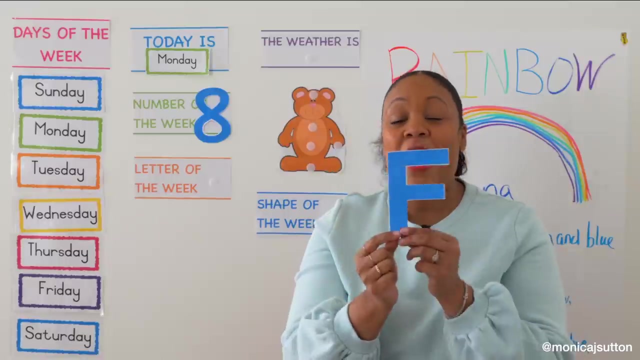 Pointer finger up, Go down, Across on the top, Across in the middle. Stop, That is letter F. F says F, F, F, F. Every letter has a sound And F says F. Thank you, That's letter F. 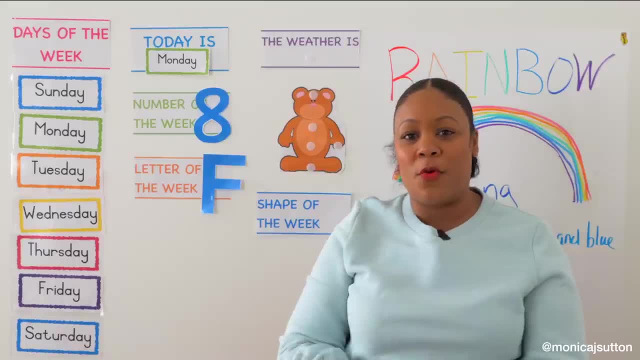 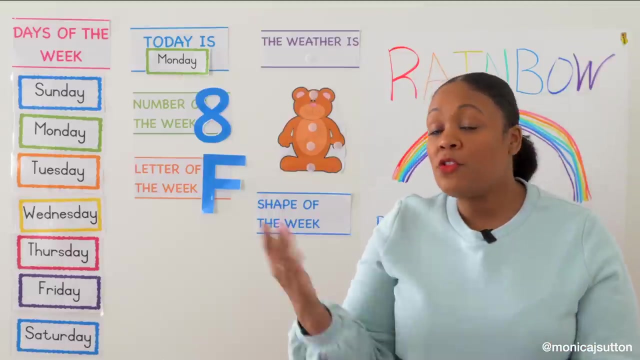 Okay, Letter F back on the board. Now we have to look outside today, Look outside our window, And we have to determine what the weather is today. What is the weather like where you live? If you look out your window, can you see what the weather looks like? 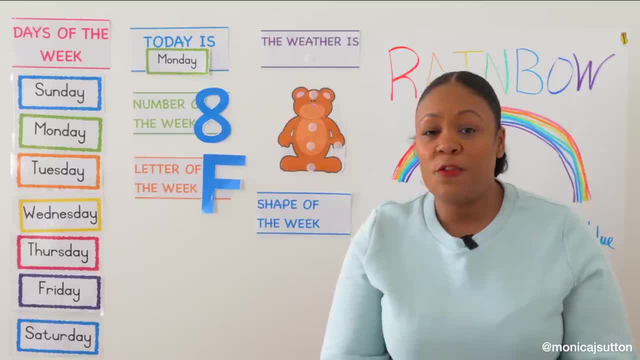 What does it look like If you use those looking eyes? what does the weather look like? Does it look like it's a sunny day? Does it look like it's raining? Does it look like it's raining? Does it look like it's snowing outside? 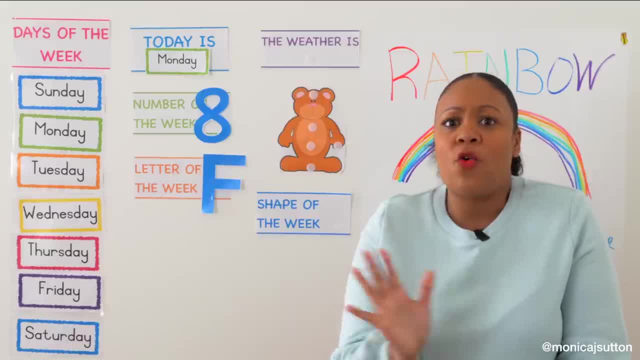 Does it look like it's snowing outside, Or does it look like it's cloudy outside? Or does it look like it's cloudy outside? What does the weather look like Just by looking with your eyes? If I look with my eyes, out of my window? 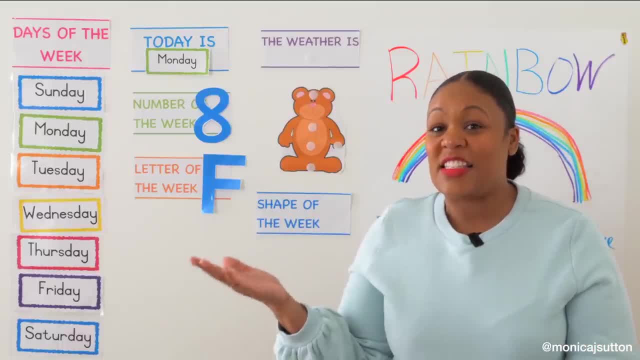 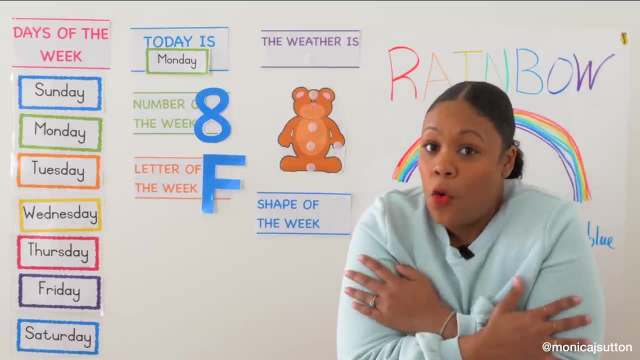 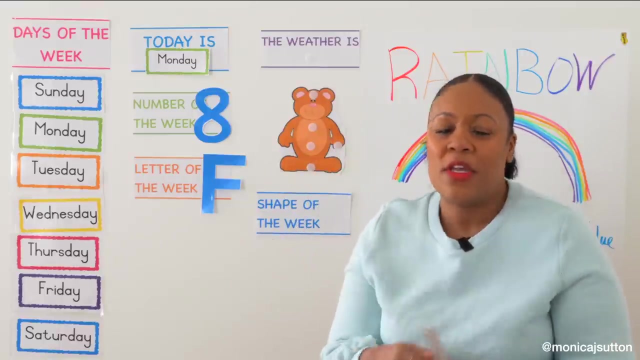 where I live, the weather is sunny. It's a sunny day, But I also know, because I went outside, that it is very, very cold today, that it is very, very cold today. The sun is shining, but it's cold. 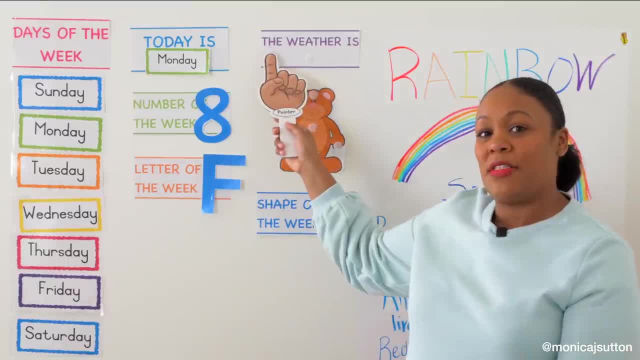 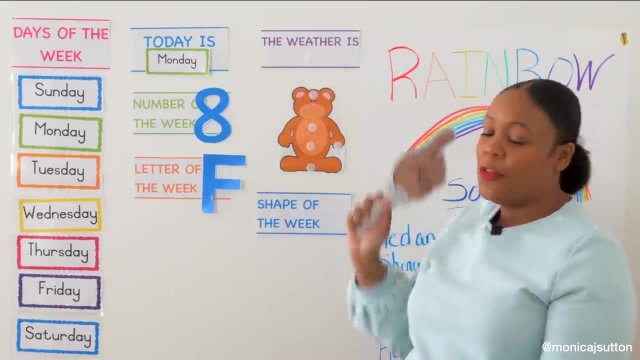 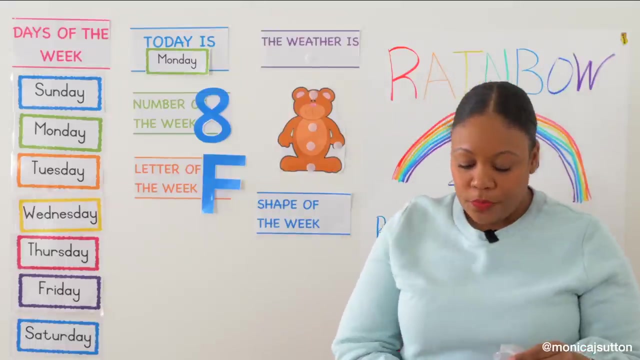 So let me see if I have a picture that can help us describe what the weather looks like and feels like The weather is. Let me get my pictures. Here's my little bag with all my weather pictures. So I'm going to open up my little bag. 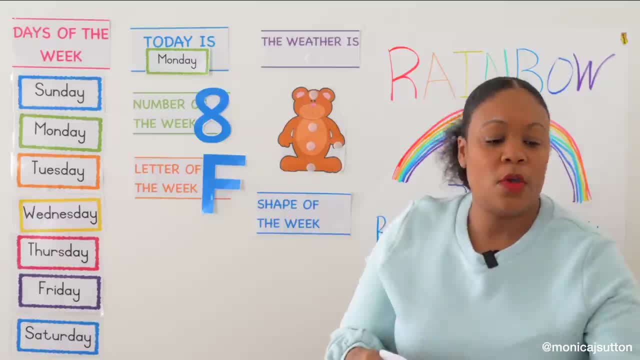 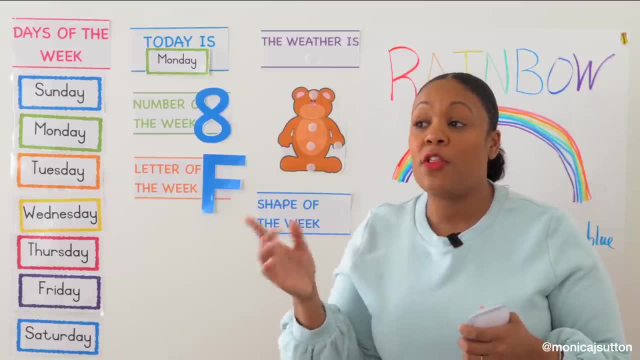 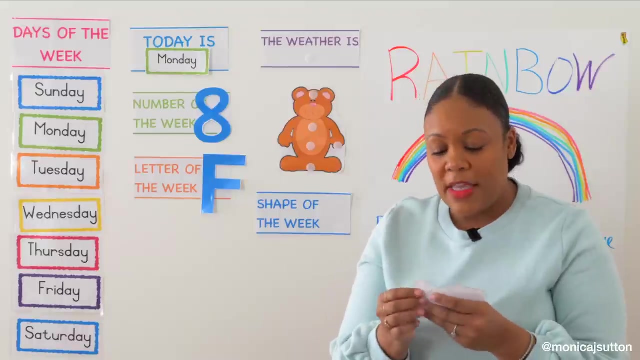 with all my weather pictures, And let's see which picture describes the weather today. Now remember where I live. where I live, the weather looks sunny, Really sunny. The sun is shining bright, But it's very cold outside. So let's see if we can find. 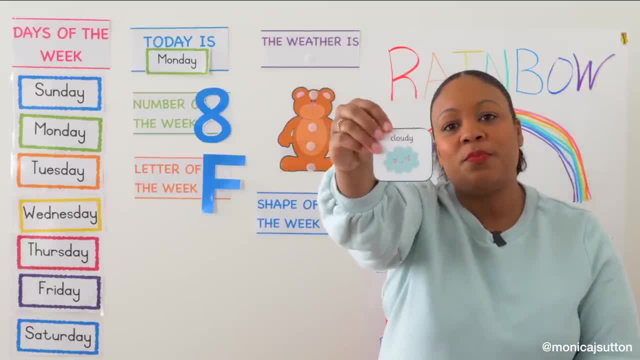 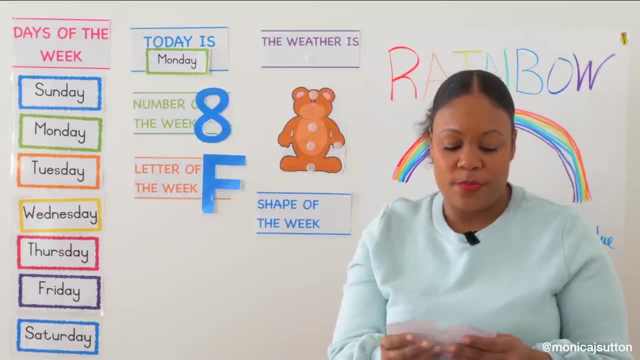 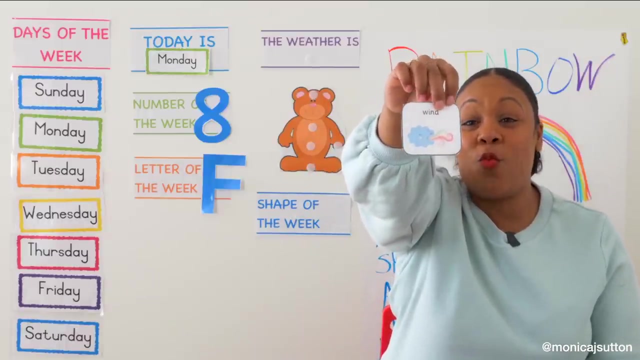 a sun picture? Does this look like a sun picture? Nah, This is cloudy. How about Let's see This one? Oh, This picture is a picture of wind Or windy, But it's not windy. out I see a lot of sun. 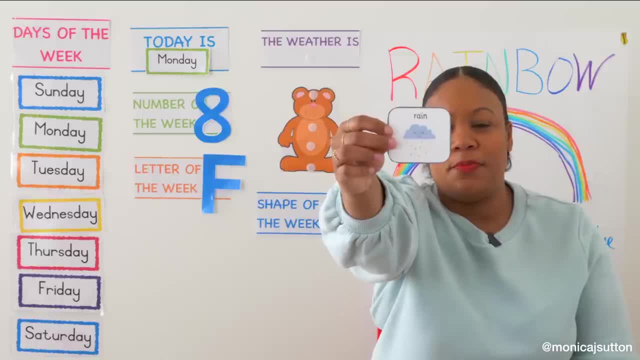 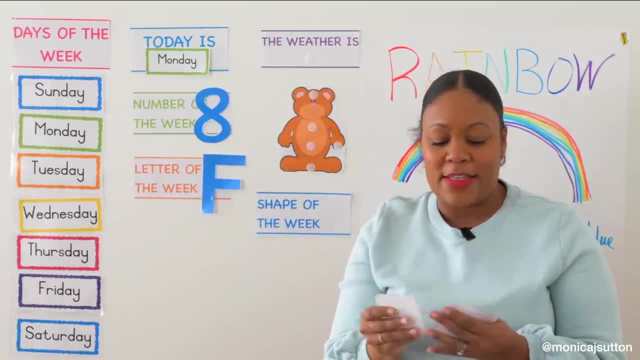 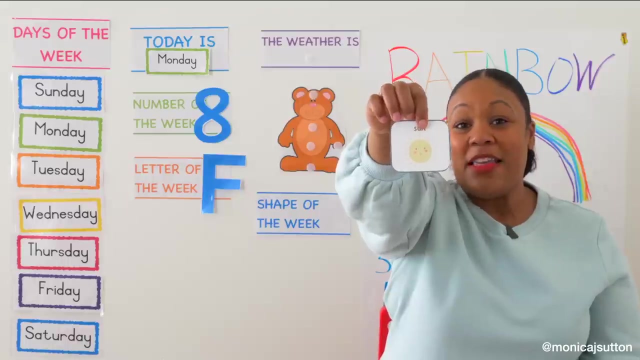 It's really, really sunny. How about this picture? What do you think? Oh no, This is a picture of rain. It's not raining out, Not today. Today is sunny, So let me see if I can find it. Yes. 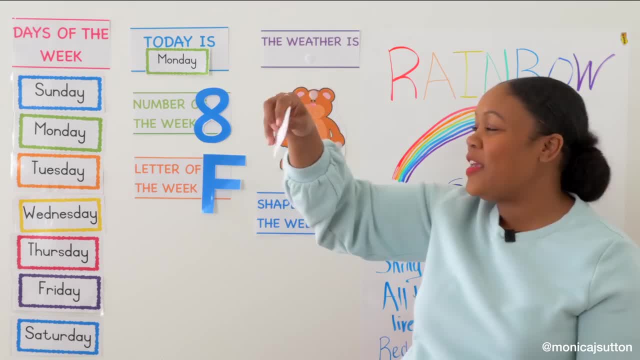 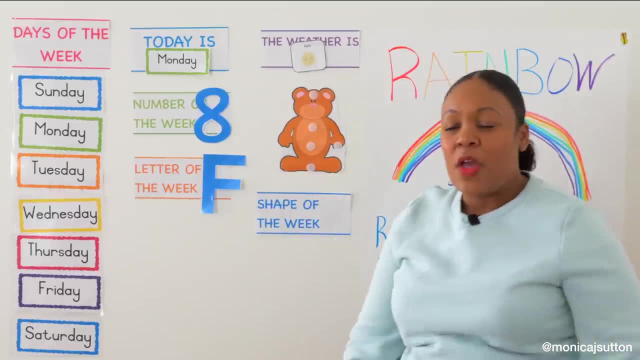 This is a picture of the sun, And since it looks sunny out, the weather is sunny- We're going to put a picture of the sun Now. let's read this together. First I will read it, Then we'll read it together. 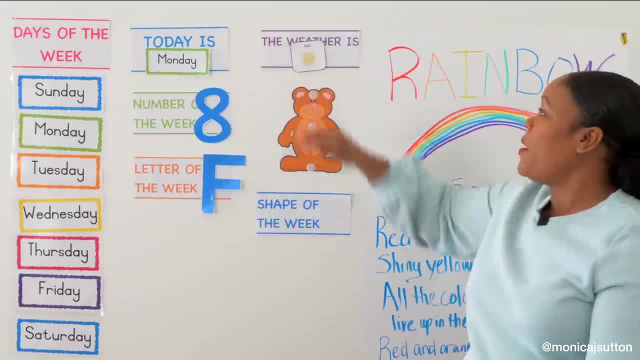 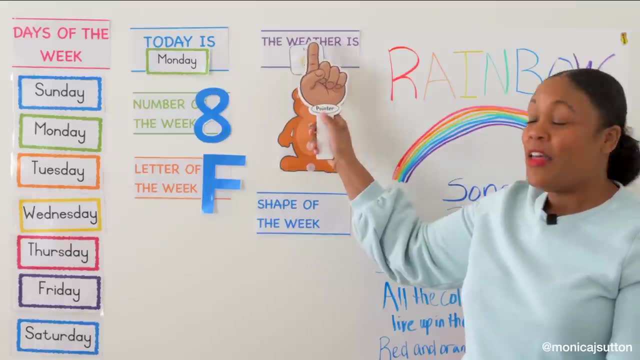 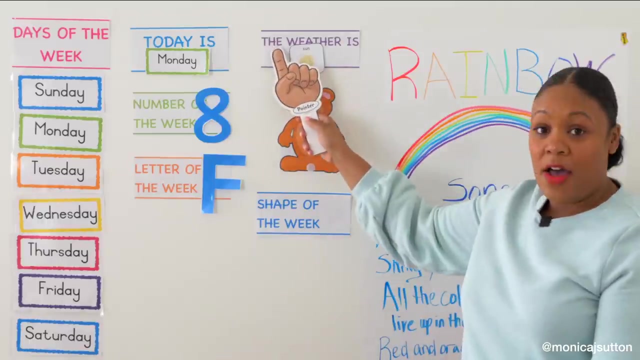 Okay, The weather. Oh, let me move it down a little. Can you see that The weather is sunny? The weather is sunny. Can you see that? Can you read it now with me? Let's do it together. The weather is sunny. 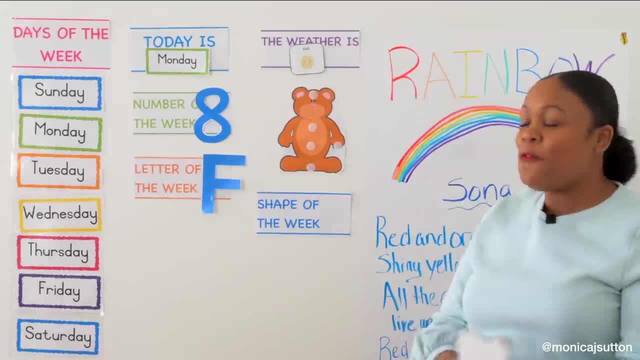 The weather is sunny out And my friend, Mr Weather Bear- This is Mr Weather Bear. He is not wearing any clothing yet And he needs us to help him get dressed for the day. And it's sunny out, We know it looks sunny. 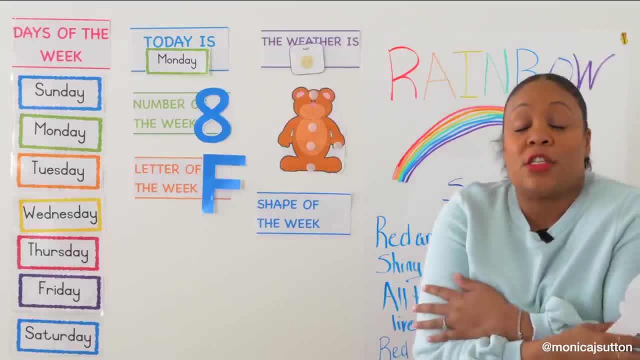 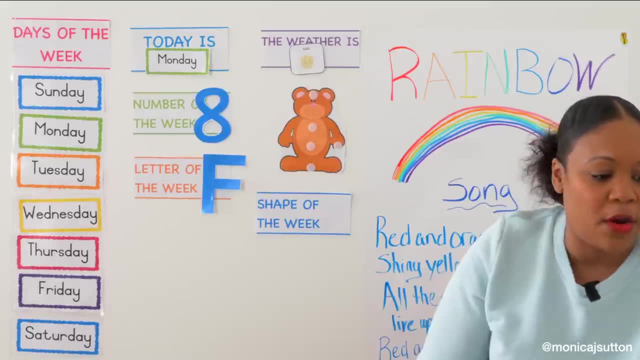 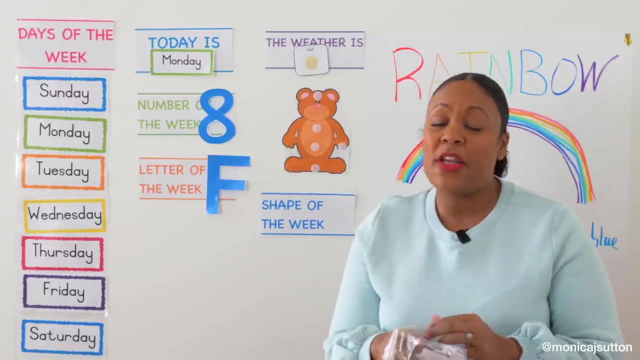 And I also told you that it feels cold. It's sunny And it feels cold, So what can we dress Mr Weather Bear with? I have a bag with Mr Weather Bear's clothes in it. Now remember, we said it looks sunny out. 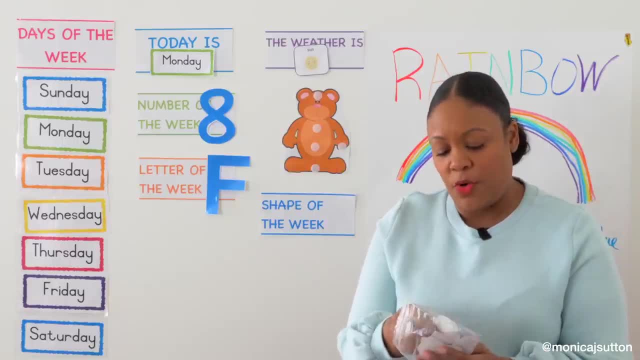 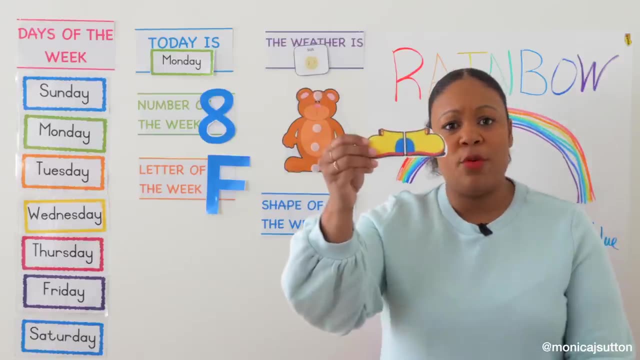 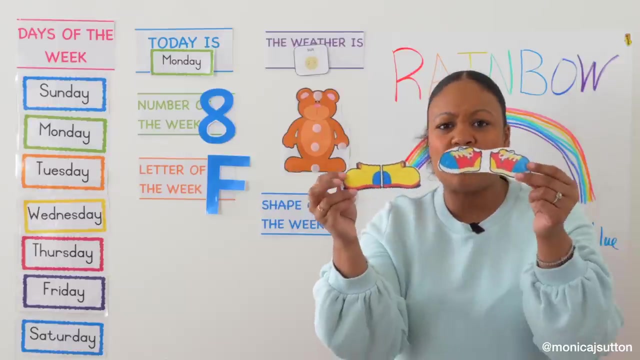 But it feels really, really cold. So let's see what we should put on Mr Weather Bear's feet. It's sunny and cold. Should we put on rain boots, Or should we just put sneakers? It's not raining out, It's sunny and cold. 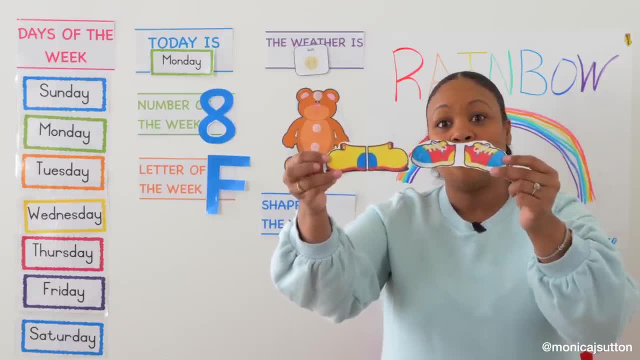 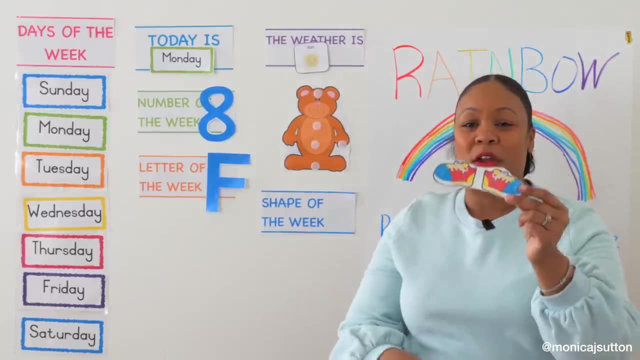 Do you think Mr Weather Bear should wear rain boots or sneakers? If you said sneakers, I think I agree with you. We can put sneakers on Mr Weather Bear. Let's put on his sneakers. Alright, Mr Weather Bear, There go your sneakers. 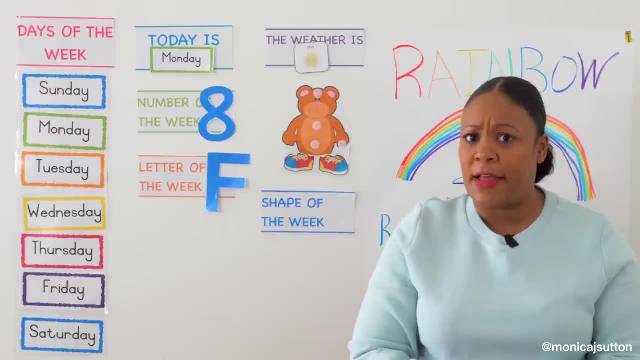 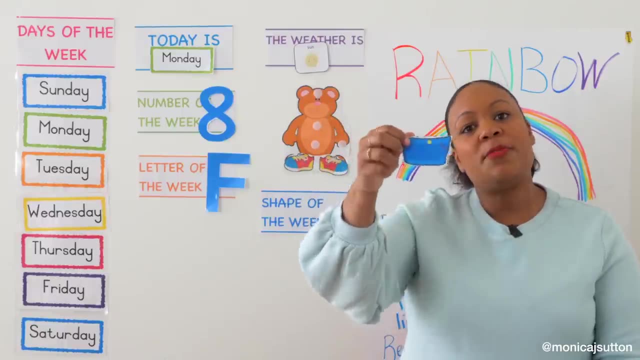 Now Mr Weather Bear has to wear some pants outside. I'm wearing jeans today And I have some jeans for Mr Weather Bear, So let's put some jeans on Mr Weather Bear, Because he can't wear shorts outside, right. 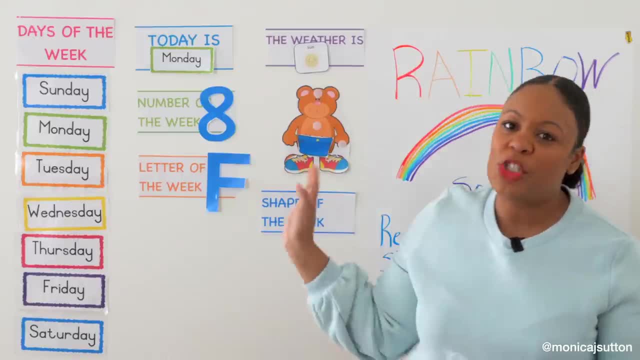 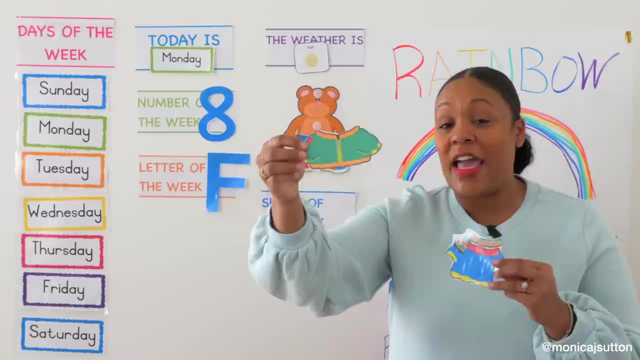 It's too cold. It's too cold for shorts, So we're going to put jeans on. Mr Weather Bear. Now we said it was cold outside, So should we put on a light, light jacket, Or should we put on a coat? 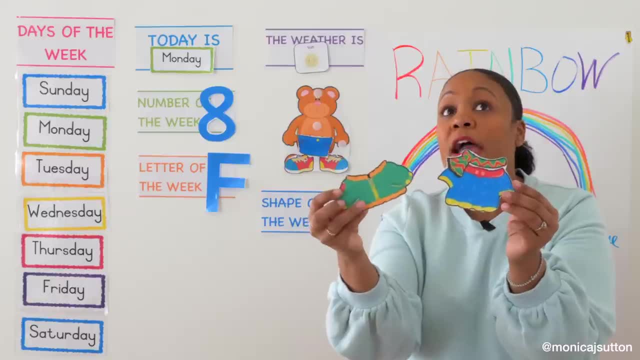 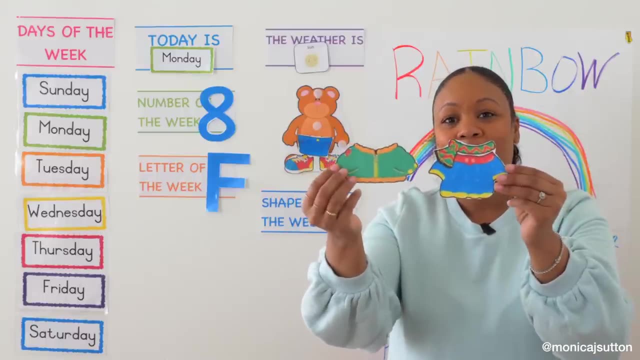 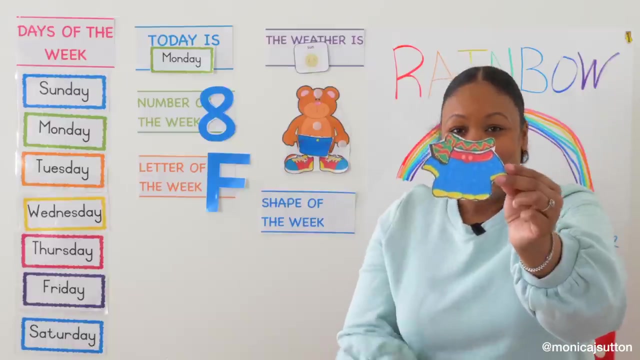 with a scarf for Mr Weather Bear. If it's cold outside, do you think he needs a light jacket or a coat with a scarf? If you said a coat with a scarf, I think I will agree. Let's put on the coat with the scarf. 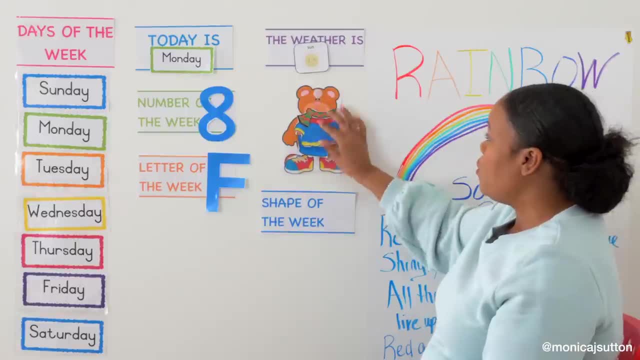 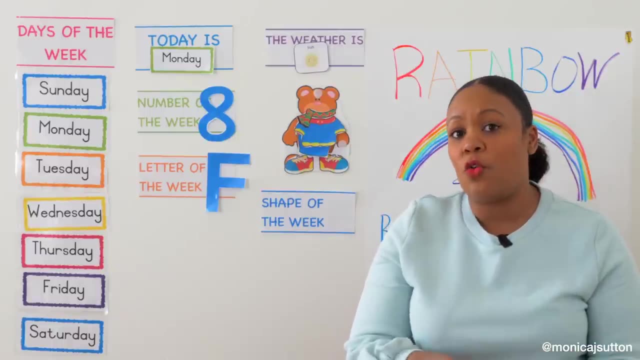 Okay, Mr Weather Bear, We're going to put on your coat and scarf so he can stay nice and warm outside, because it's cold outside. And since it's cold, maybe we should put something on his head. That's right on his head. 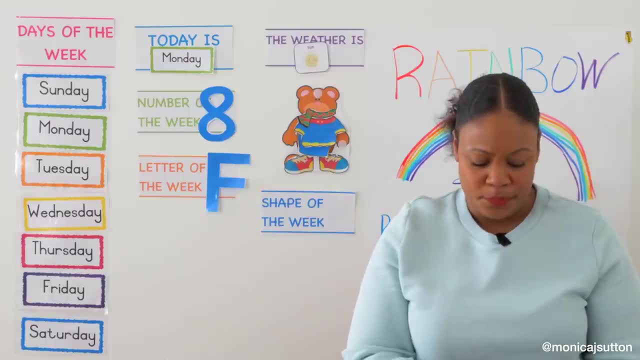 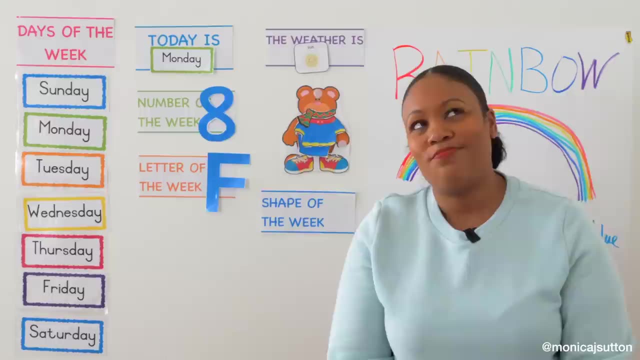 What should we put on his head? You tell me What should we put on his head. Should we put an umbrella on his head? Nah, We don't need an umbrella. It's not raining. Should we put a? I don't know. Should we put sunglasses? 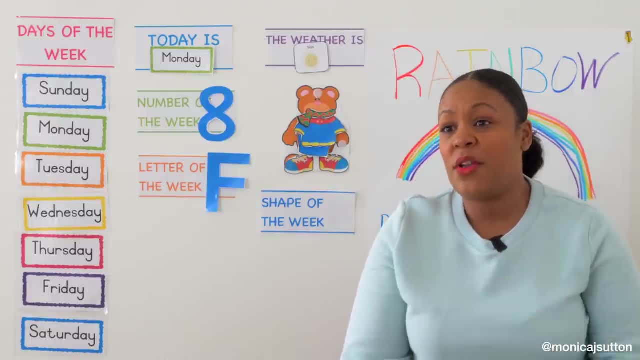 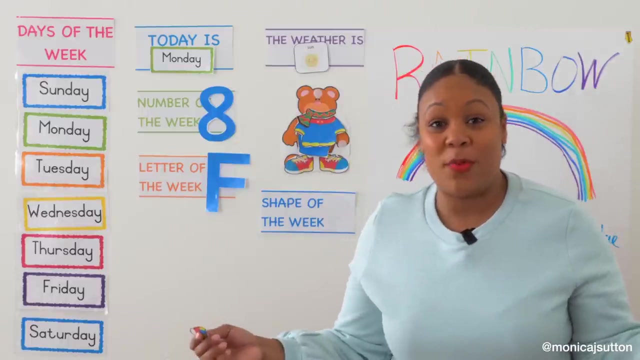 on his head. Well, it is a little sunny out, But what will keep his head warm? Will the sunglasses keep his head warm? No, But I have an idea. Hmm, Maybe a hat. What do you think? Should we put a hat? 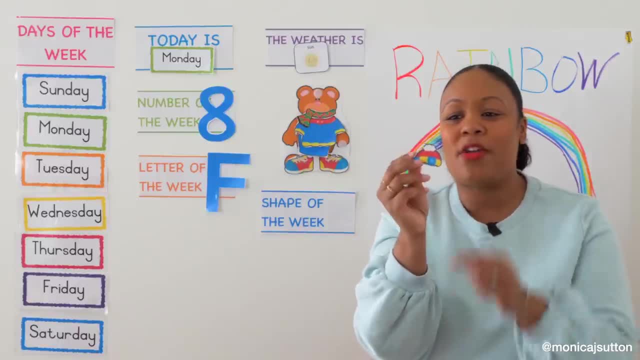 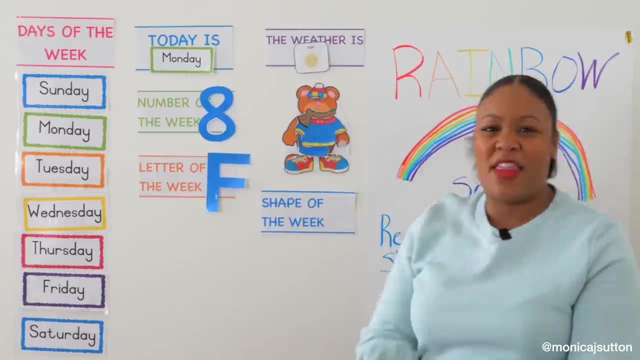 on his head. I have a little hat for Mr Weather Bear, A winter hat with a pom-pom on top, Do you agree? Good, Let's put on his hat. Oh, Mr Weather Bear, that's a small hat, right. 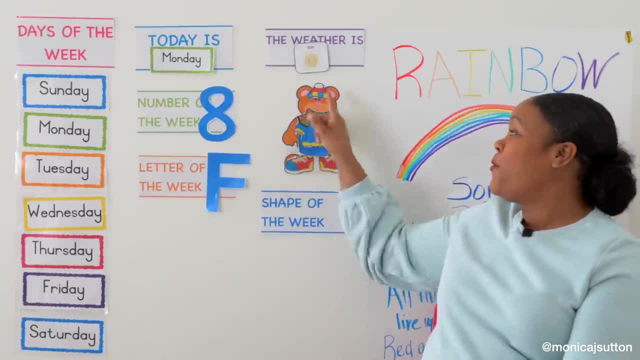 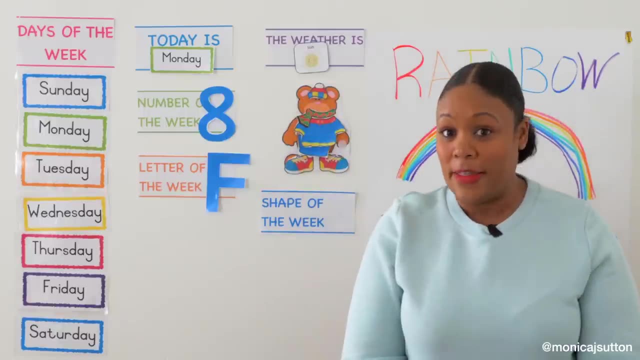 We're gonna have to get a bigger hat for Mr Weather Bear, But for now I think that'll work. Maybe we can make a hat for Mr Weather Bear that will cover his ears too. What do you think? Do you think we should make a new hat for him? 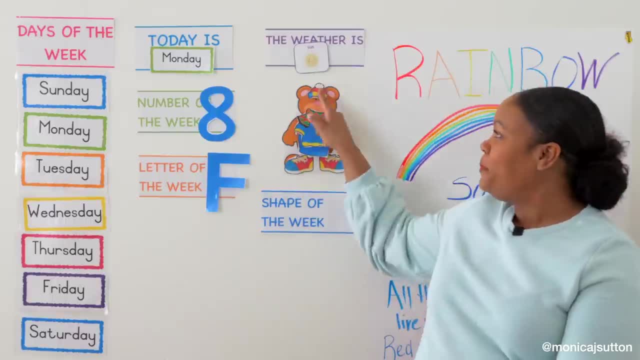 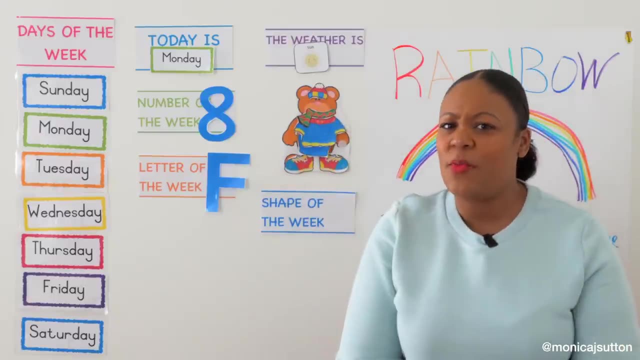 I agree. I think we should make a new hat for Mr Weather Bear, But for now that's okay. So he's wearing a hat, scarf, a coat, some jeans and some sneakers. I think he'll be nice and warm. 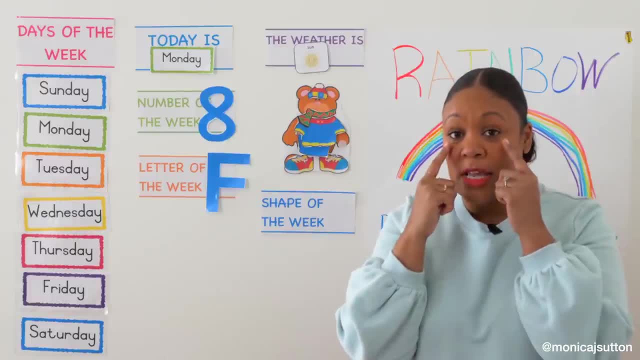 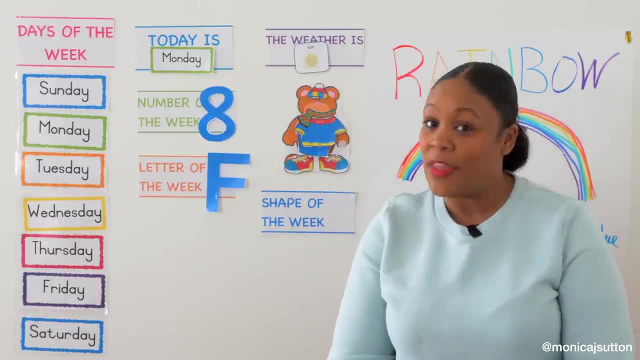 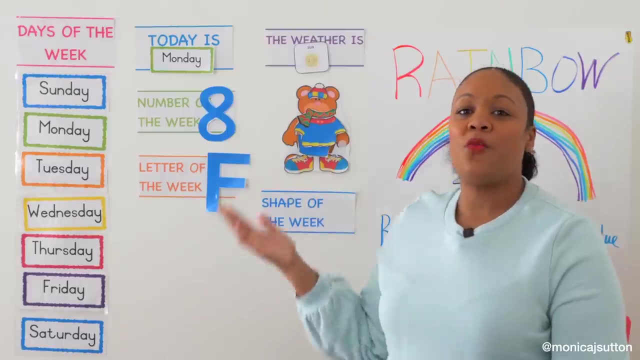 And ready to go outside. Remember, the weather looks sunny but it also feels cold. So I think Mr Weather Bear is ready to go. You think so, I agree. Now, the last thing I want to go over is our Shape of the Week. 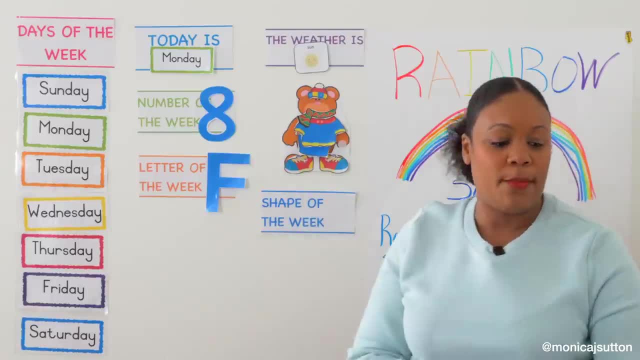 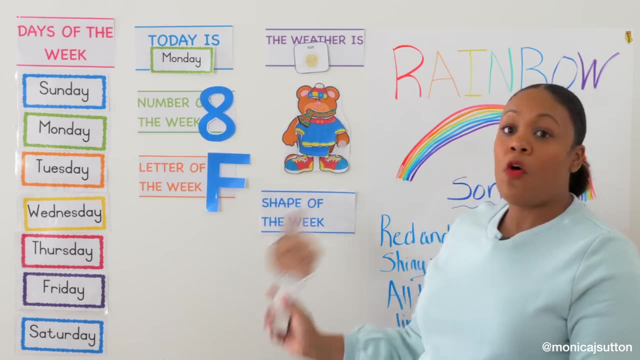 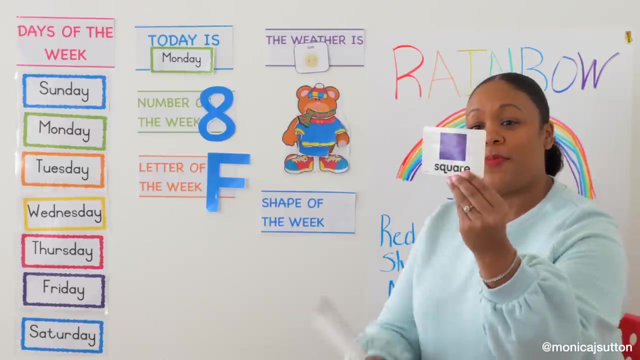 Let's read it together: Shape of the Week. Oh, I'm missing my pointer Pointer. This pointer helps me to point to all the different things on the board. So Shape of the Week, Shape of the Week, Our Shape of the Week is: 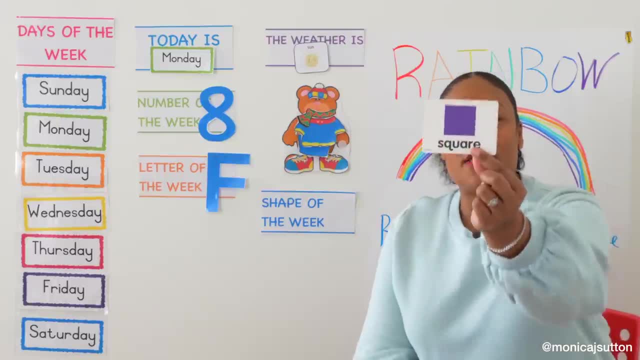 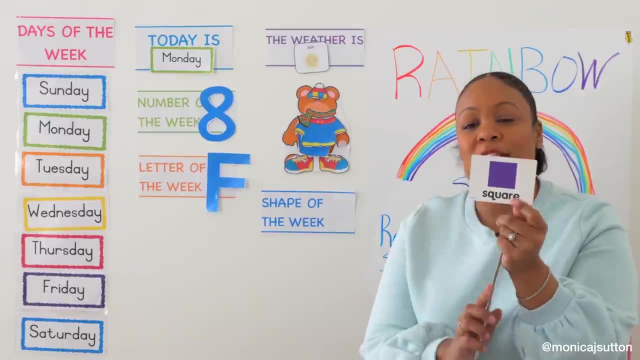 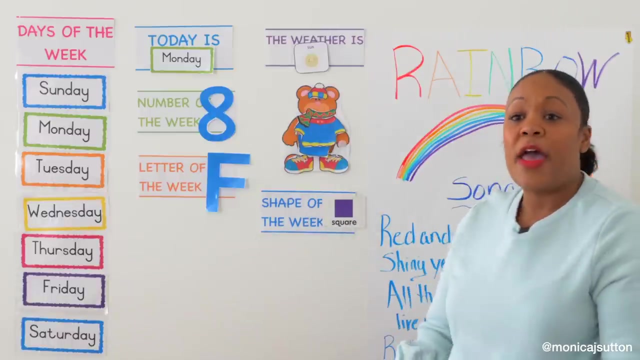 the square. The square is our Shape of the Week, And what makes the square so special is that it has four sides. Four sides, Let's put the square up. The square is our Shape of the Week. Help me count the sides of the square. 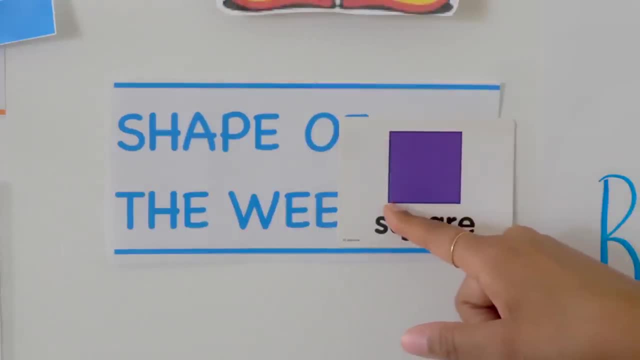 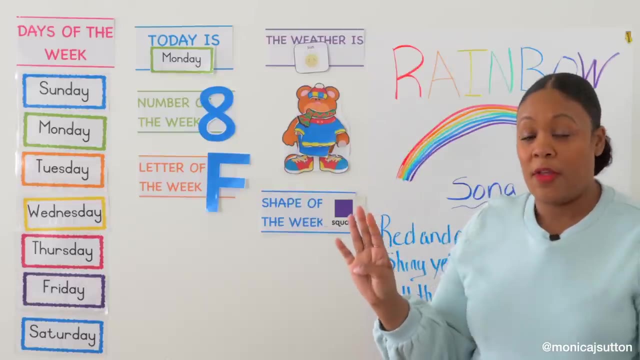 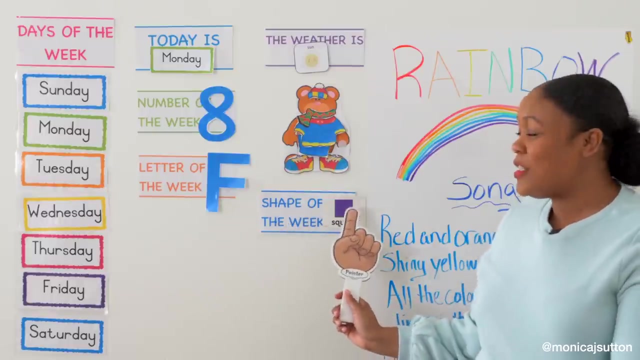 One, two, three, four. One, two, three, four, Four sides on a square. There are four sides on a square, That's right. So our Shape of the Week is the square. Our Letter of the Week is F. 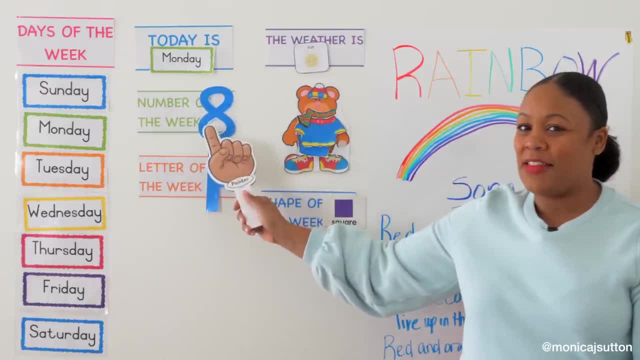 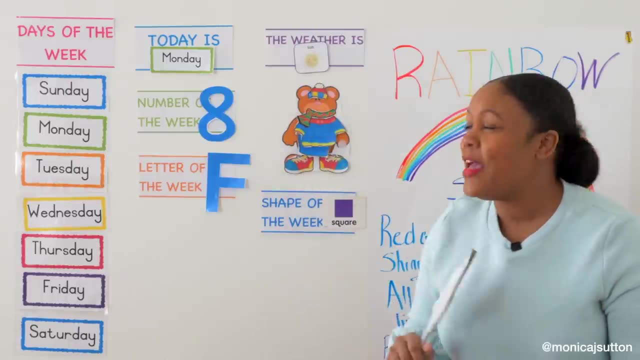 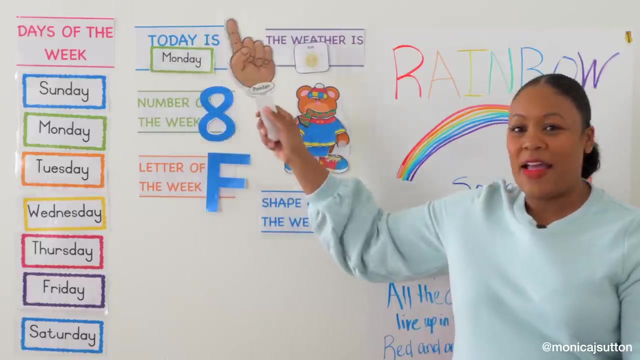 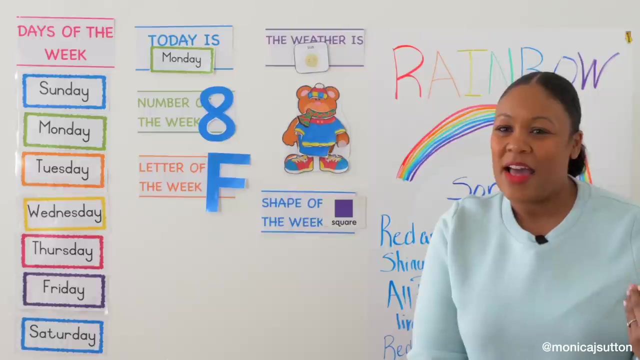 Our Number of the Week is number eight. And we said, the weather today is sunny but it feels cold, And today is Monday. Today is Monday. Thank you all for joining me for our Circle Time. Circle Time with Miss Monica. Now, before we go, 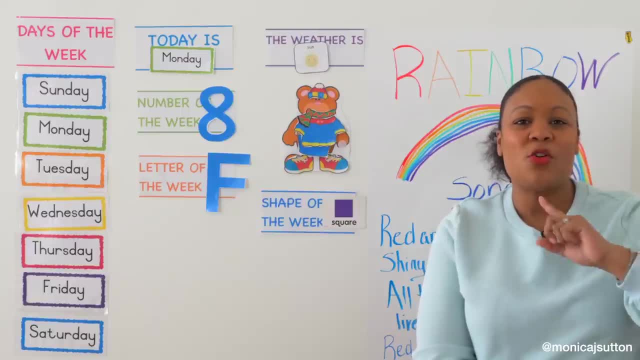 I think we should end with one special song. So we need to go to our song bag. Here's our song bag And we need to pick a song for today. Let's see what song comes on top. Oh, Look at what song's on top. 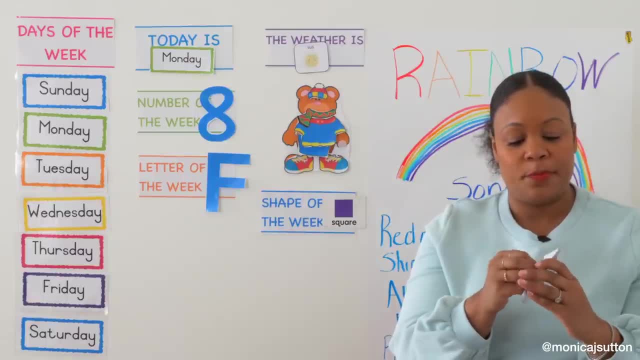 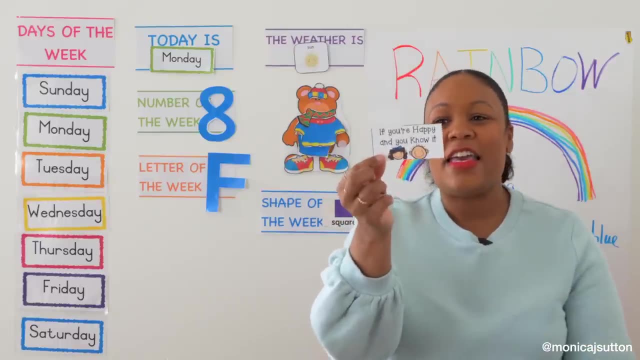 Dun dun. This is our song for today. Oh, let's pick it up. Okay, come on. song of the day. Our song of the day is: If You're Happy and You Know It, That's our song of the day, So you can help me. 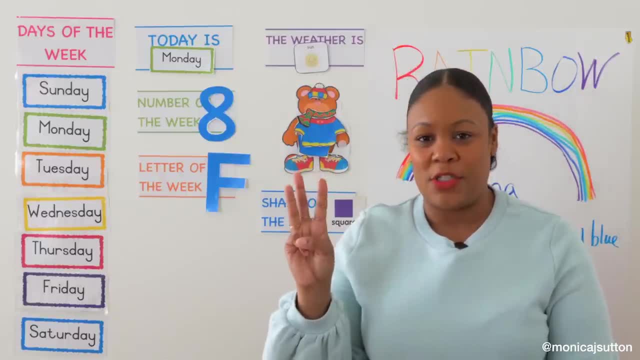 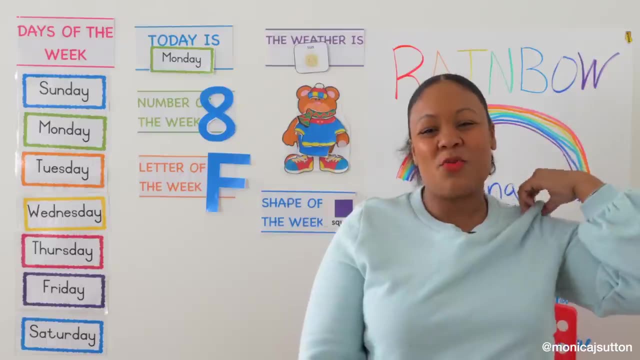 sing, We'll do three different actions. We'll clap our hands, we can stomp our feet and we can shout hooray. Okay, So those will be our three actions. Our three actions for If You're Happy and You Know It. 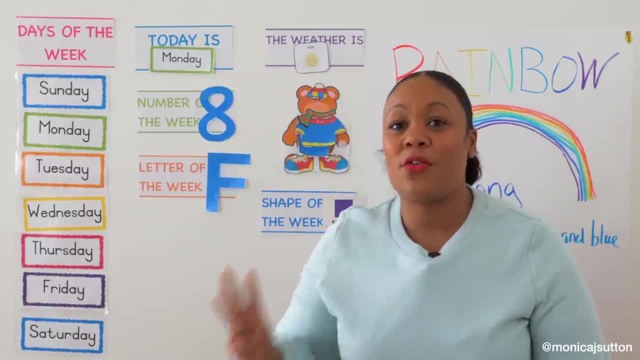 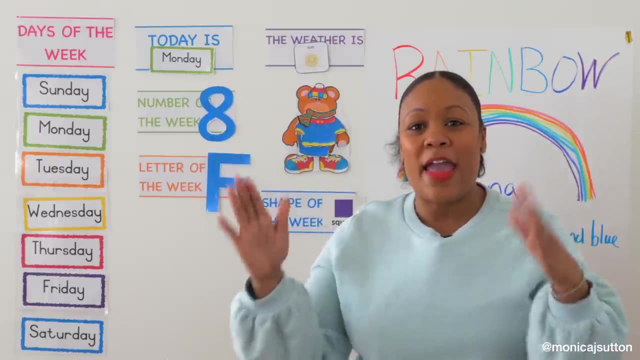 Let's start on three: One, two, three. If you're happy and you know it, clap your hands. If you're happy and you know it, clap your hands. If you're happy and you know it and you really wanna show it. If you're happy and you know it. 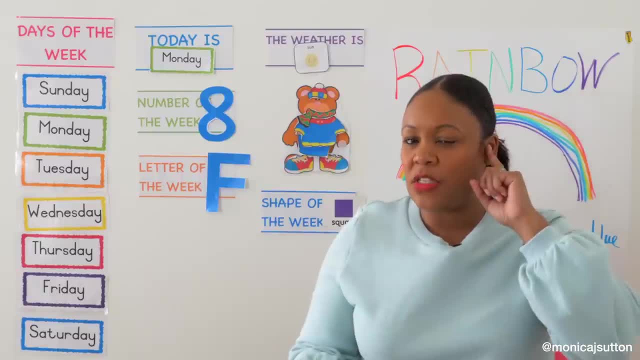 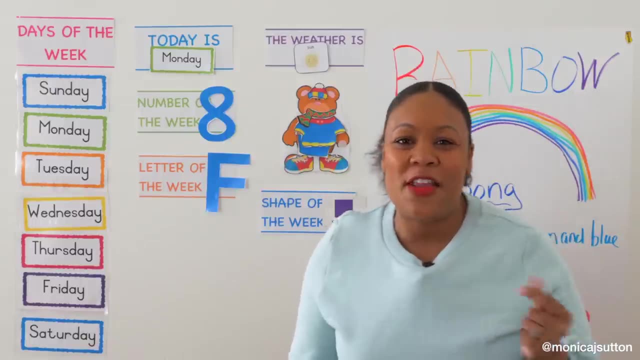 clap your hands. If you're happy and you know it, stomp your feet. Oh, listen to my feet. If you're happy and you know it, stomp your feet. If you're happy and you know it and you really wanna show it. If you're happy and you know it.